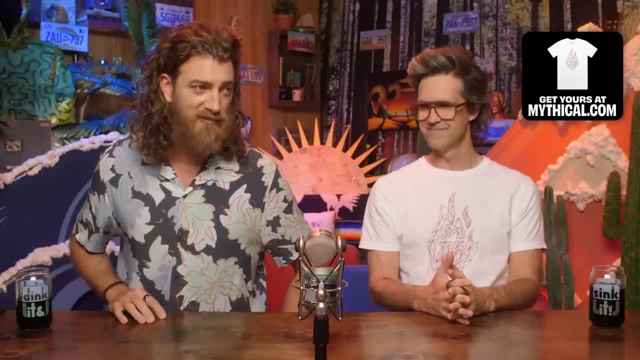 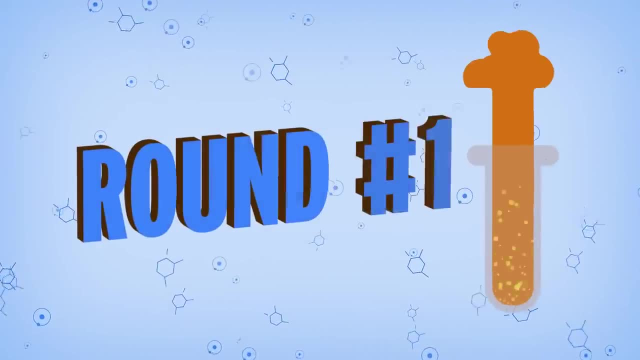 about science experiments. that would be a crap ton easier if we just used instructions. It's time for Science Without Guidance. featuring the Beaker Boys. Hello, Beaker Boys, Hello. Here's how this goes. Each round, you'll have 10 minutes. 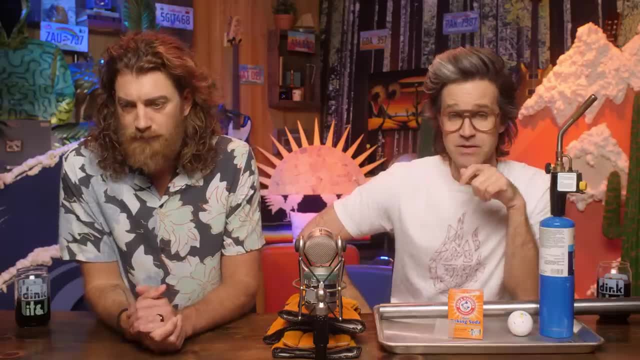 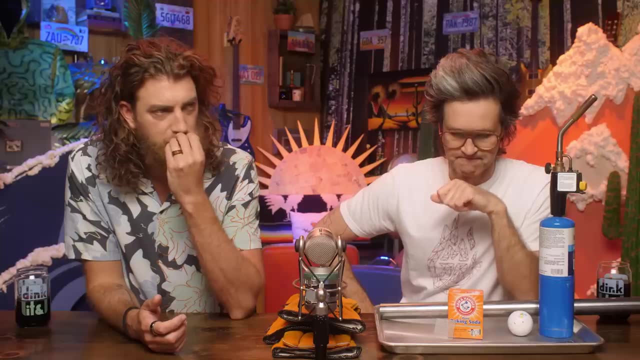 to use some combination of the items in front of you to achieve a surprising scientific result. There are some decoy items that throw you off as well, And you can use lifelines to help you along the way, but they're gonna cost you some points. 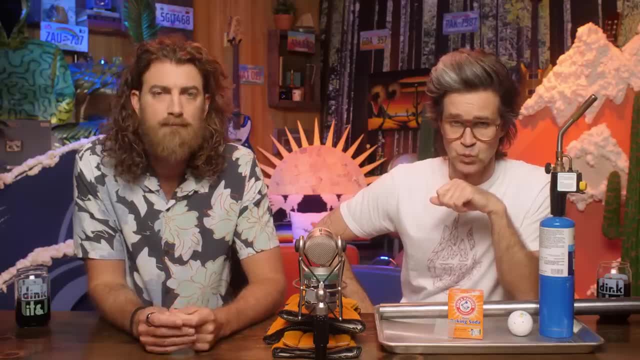 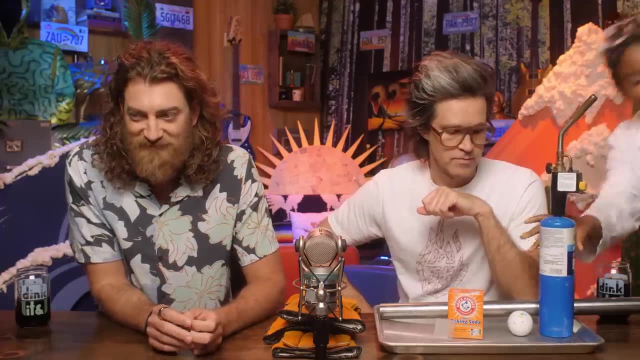 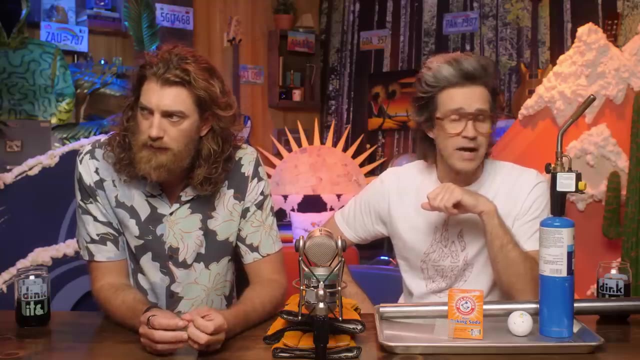 every time you use them. They are as follows: A message from Science Mykayla about a scientifical, scientifical principle at play. This costs one point. I reveal a decoy item. This costs two points per decoy item. 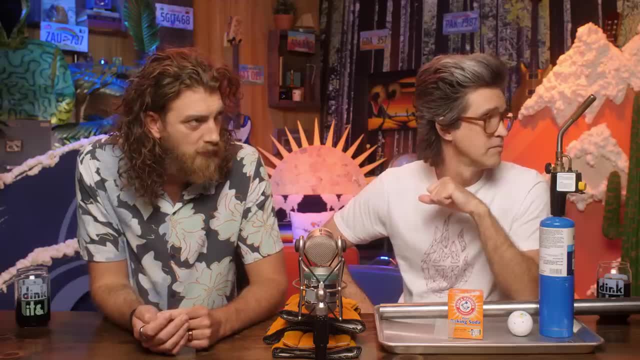 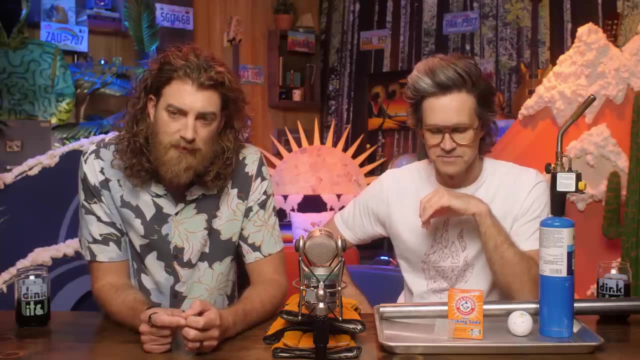 How do you feel about being cheaper than Stevie's? I'm okay with it. Okay, You're a deal, You're a steal, Yeah, Or I vaguely tell you what result you're trying to achieve, Vaguely For three points. 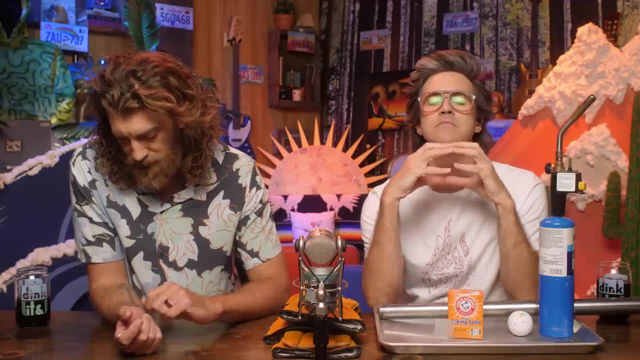 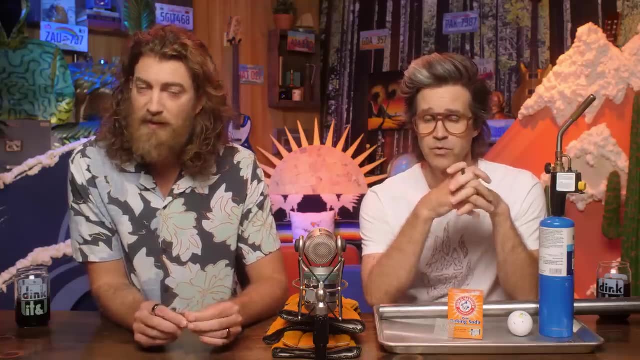 And you'll have 30 points at your disposal And if you manage not to use all of them, you will receive actual Beaker Boys As a prize. Really, Are you ready? Well, first can I just point out, we have to raise these boys. 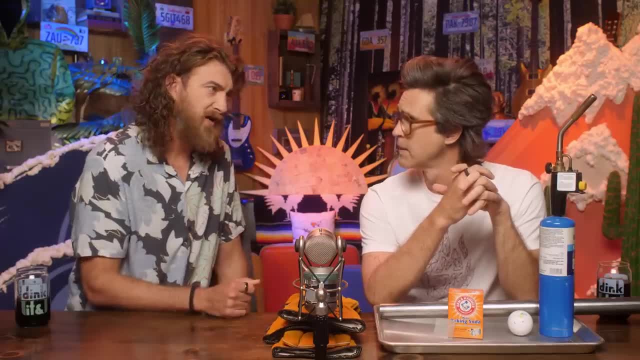 This is a lot like how actual science at a real university research universities happen. Right, They've got decoy items. Here you go. They can ask for vague hints. Oh, you want me to go ahead and glove up? I mean, they've given it to us. 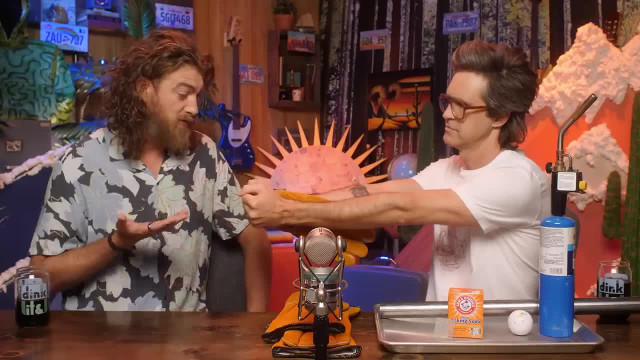 and there is this torch here and I am gonna use that. Okay, so this round has two decoy items. We're gonna put 10 minutes on the clock. Good luck, Your time starts now. All right, All right, All right. 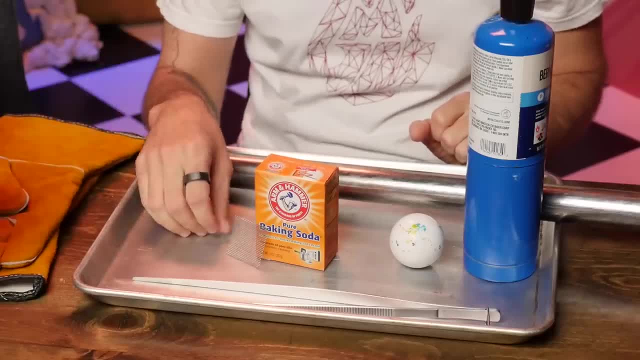 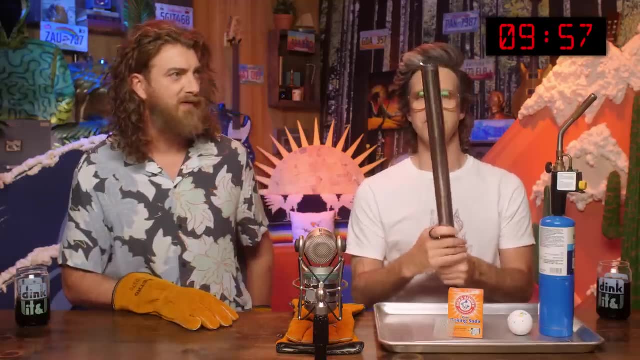 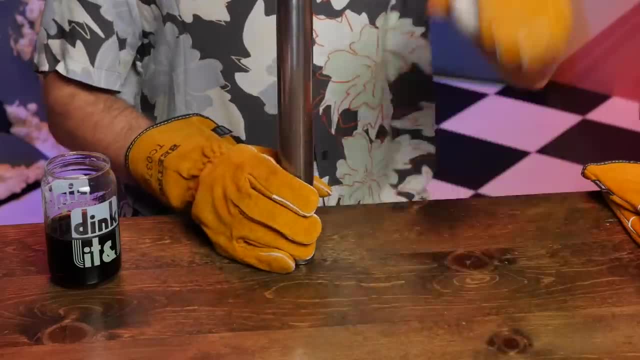 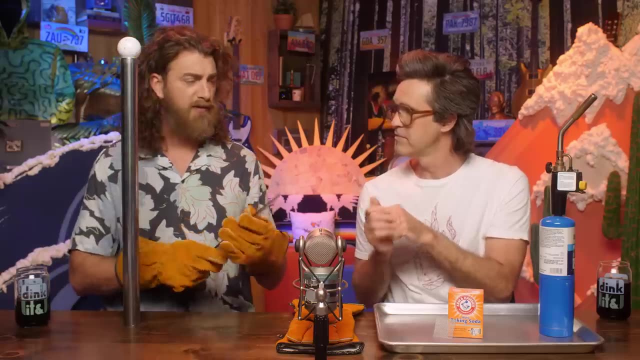 A jawbreaker Boy. you know how to do one of that. The largest set of tweezers ever Shall I? You want me to get some of the unibrow? Uh, I don't. Mine's quite grown. It looks like you've got yours. 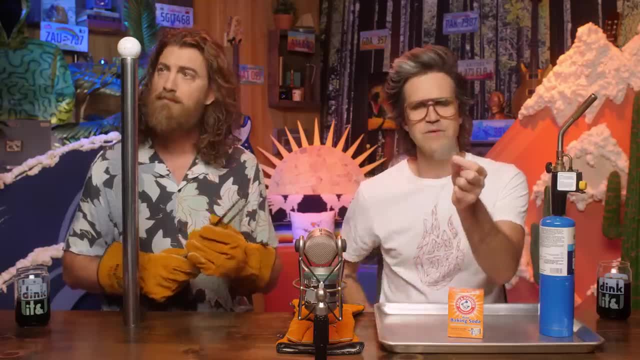 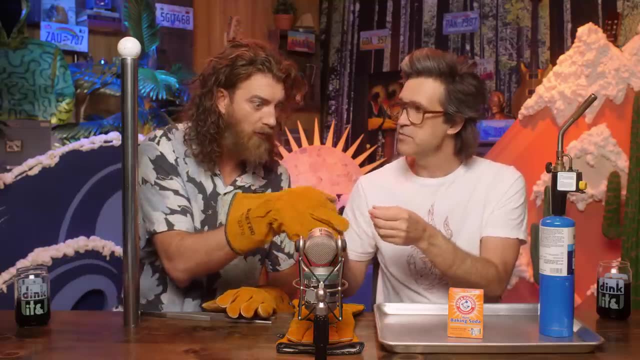 I still have to get mine. We have a little square of. It's a teeny screen for a little door. A little door, A little screen, door, A little screen, Because if you put that screen, we could put that screen on the top of the thing. 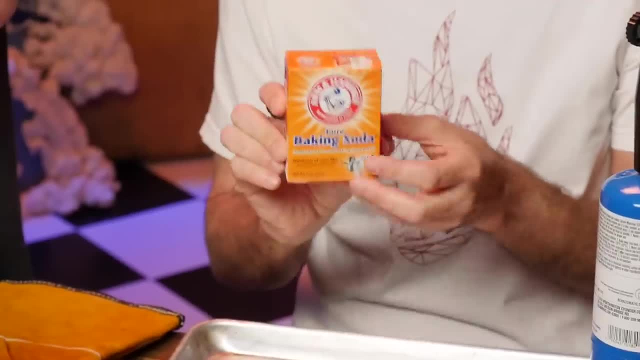 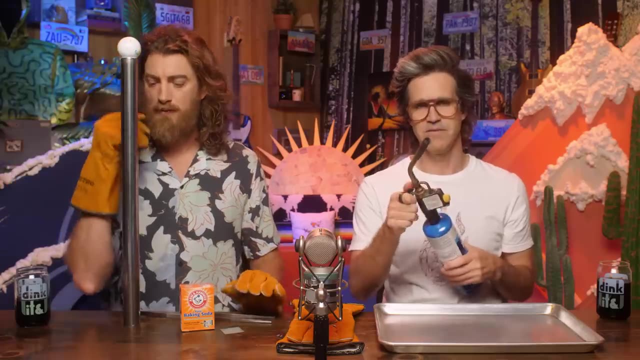 We could. And then we've got baking soda, science's favorite powder, and of course we have fire. Okay, I'm not gonna burn it all. So see, We know that the fire is not a, it can't be a decoy item. 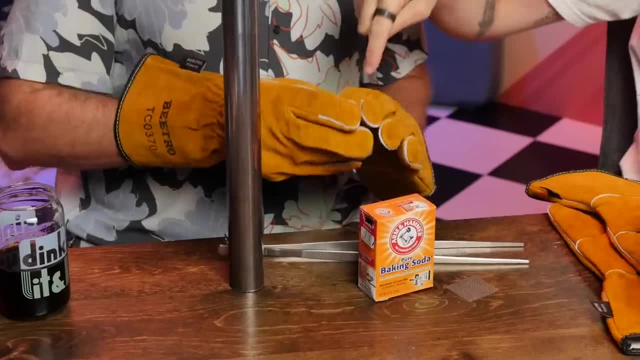 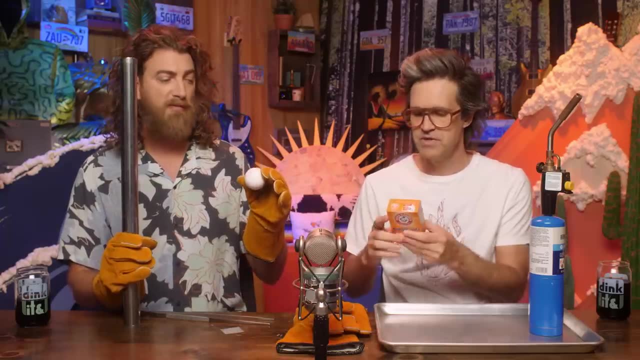 I mean, fire is too fun. Fire is necessary. We've melted a jawbreaker before. I think It's fun, Let's just. but Do you wanna do it on top of a pipe? Can you burn baking soda? What happens with that? 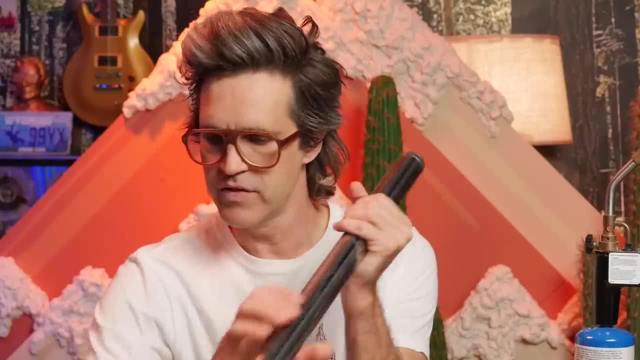 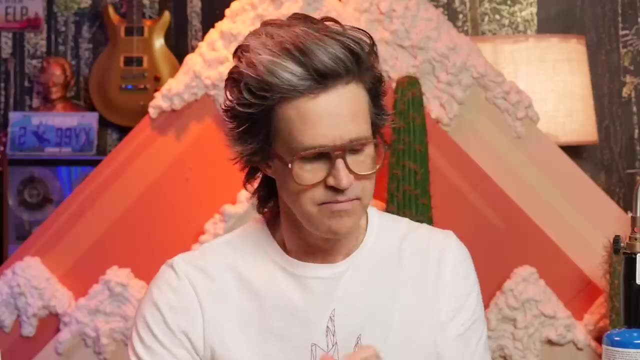 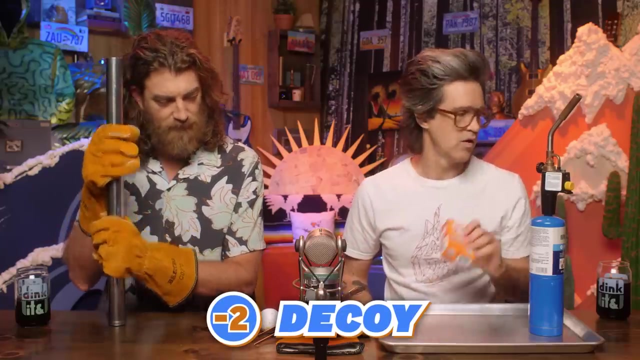 And then if you put the pipe with the screen that would like sift something, I bet you the pipe is a decoy. All right, What's the decoy item? It's expensive. You do not need the baking soda, Oh. 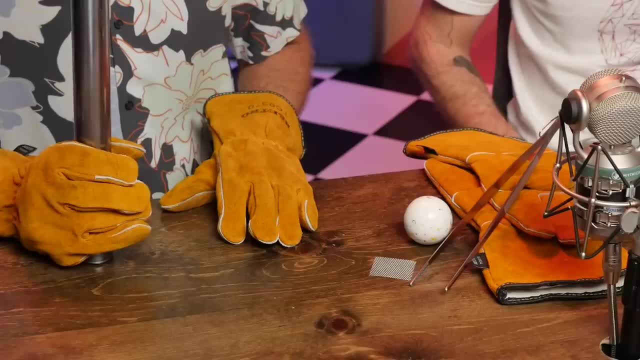 Okay. Well, there you go, All right, And there's one more of those Mm-hmm. Come on man. Okay, now we can start trying things. Yeah, let's just You wanna put it on the pipe and then burn it. 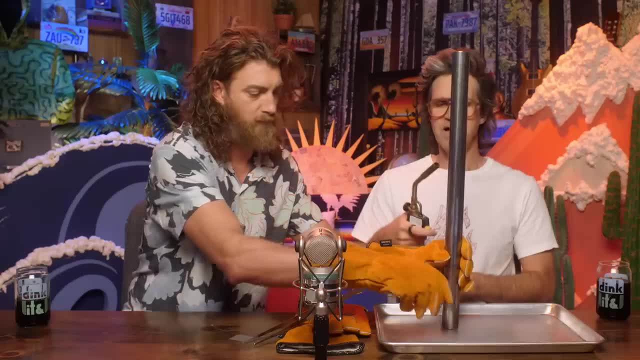 so everybody sees it. It's like a pedestal. I mean I don't wanna. if I heat up the pipe then it's gonna be hot and then I'm gonna grab it. I got gloves. I don't have gloves. 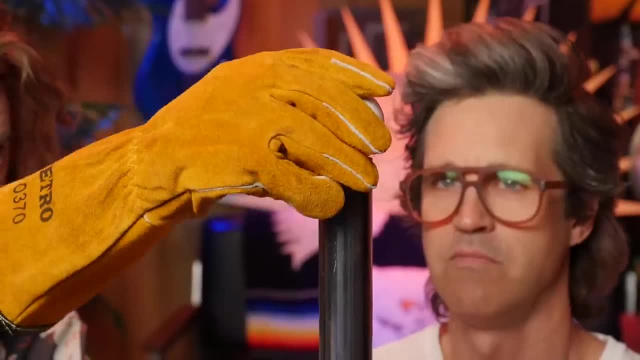 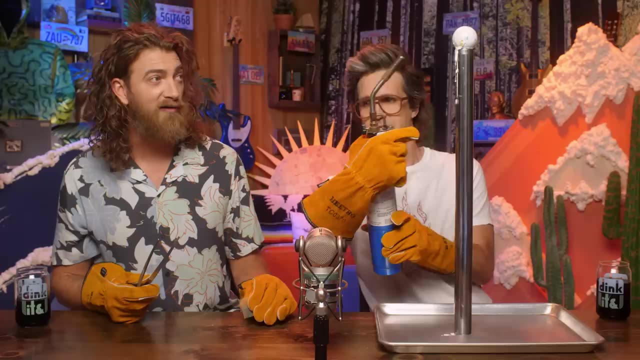 Yeah, you do. I mean I have them, but I don't have them on. Why don't you have the gloves on? Huh, See that? Well, it's fun. I don't know if it's science. That's cool. 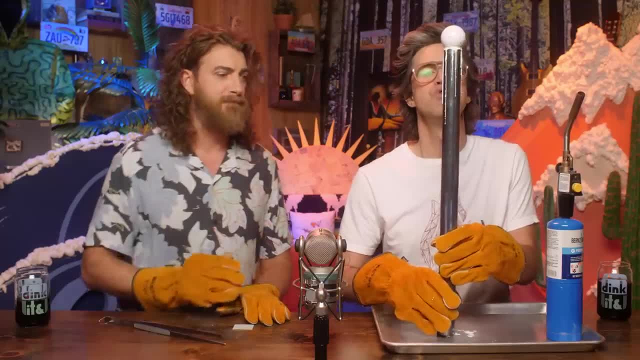 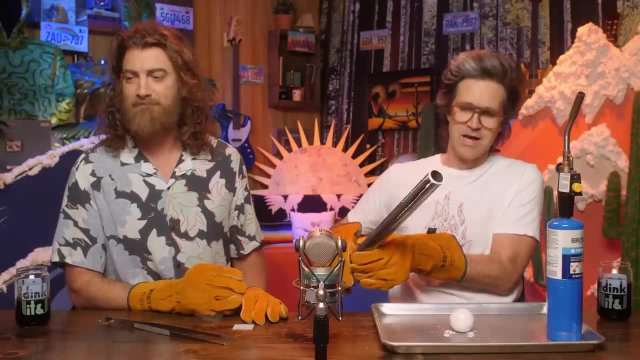 But it's fun. Now I bet you $100 if you turn that upside down, that ball's gonna stay there. That didn't work. Well, sorry, Let's bring Mikaela in. Come on, she told me to wear gloves. 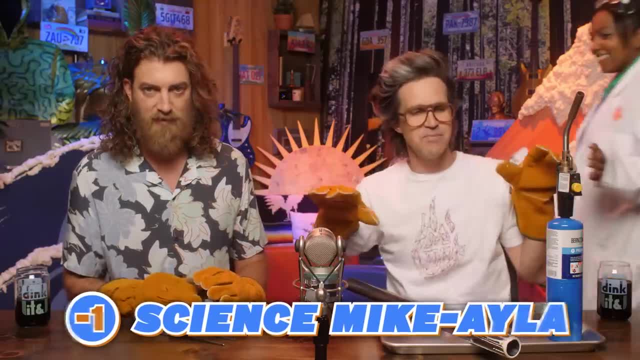 Okay, She's so helpful. It's only one point. I'm not saying she's cheap, but I'm saying the hint is cheap. Okay, I think you're saying I'm cheap. It kinda feels that way. Okay, I'm sorry. 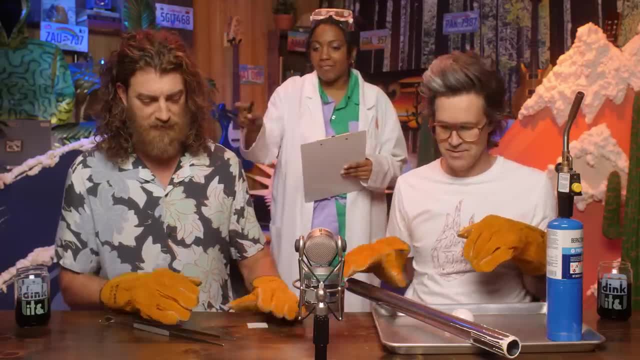 You're a steal. I didn't say it, I didn't. I appreciate you. You never insult me, That's true, And I love you for that. Maybe it's just that it's true. We should've done it this way. 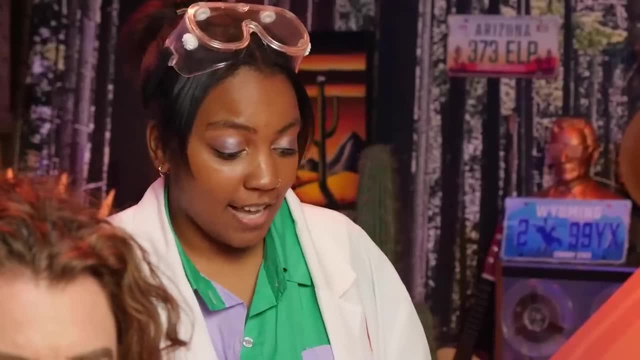 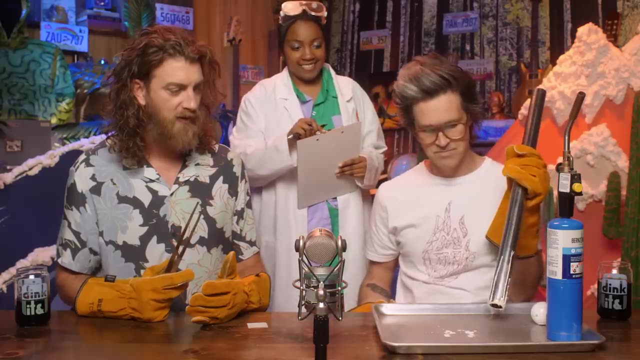 All right, you ready, She's here, Let her do her job. Okay, Acoustics and thermodynamics have been known to work together in great harmony. That wasn't harmonious, Okay. Okay, The tube is necessary. Thank you, Mikaela. 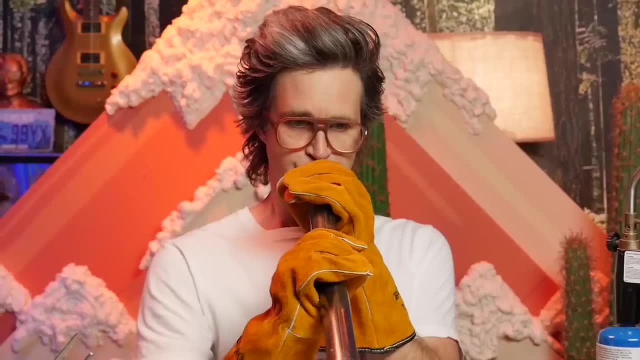 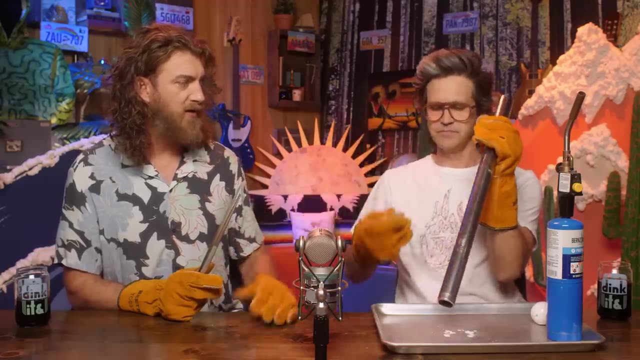 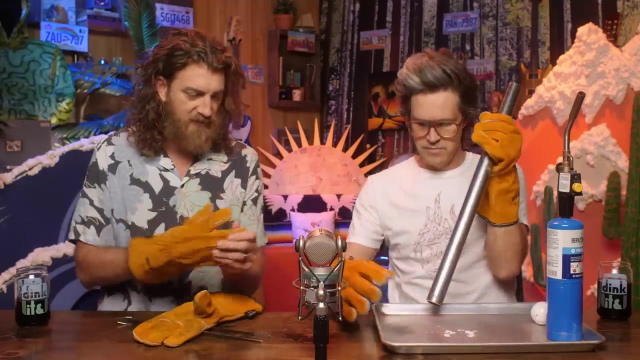 You're welcome. We're going to be making a noise, All right, so Sound. So what we need to do? Link. is you Not with our mouths? probably Put that You're making like a reed. What if you take this? what if you take this? 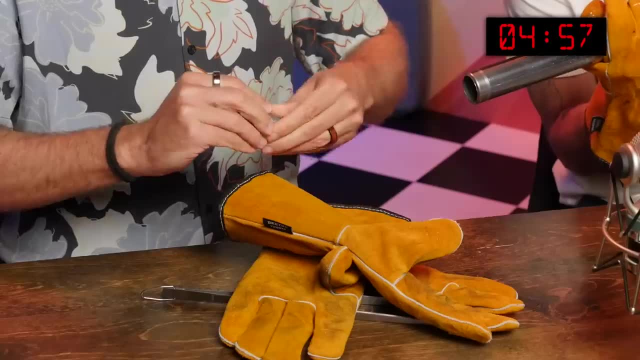 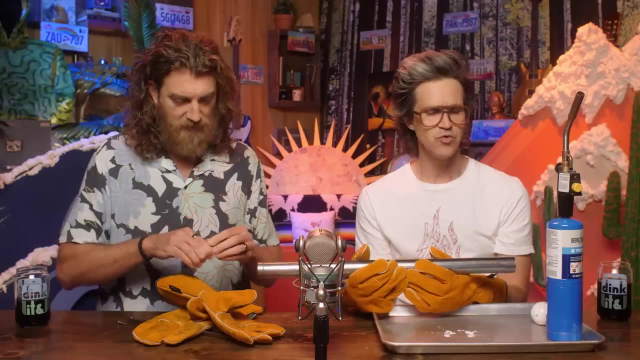 and you turn. Less than five minutes remaining, You make this like this. so you're basically kind of creating like a I don't think we need the jawbreaker, I bet Yeah, yeah, that's what I'm saying. And can we use heat to create? 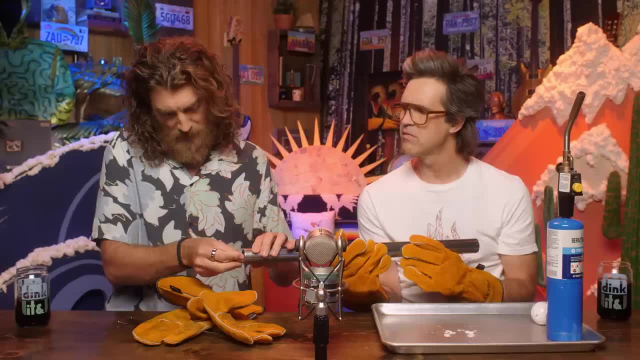 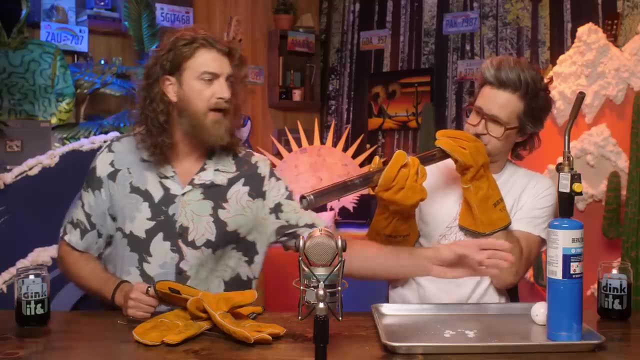 Yeah, what you're gonna do is- I'm putting this in there. it's making like a I don't know what it's doing. That doesn't seem like it would be doing anything. Blow into it like a trumpet. Yeah, yeah, yeah, yeah, yeah. 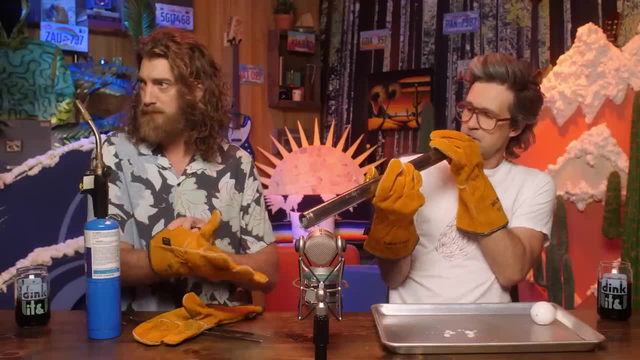 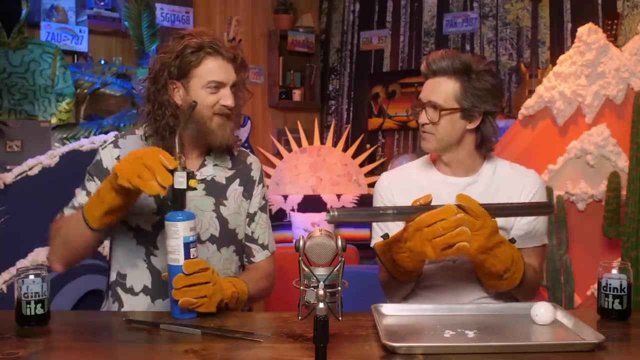 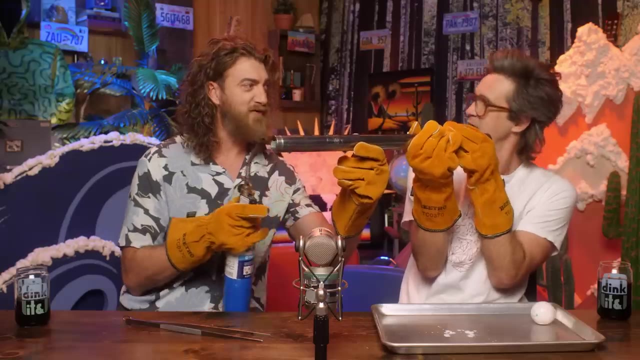 Now, as you blow into it, Okay, As you blow into it, I'm gonna heat the pipe. We've got Chappy, our resident photographer, telling us: no, Oh, is that you or the heat? I don't know. 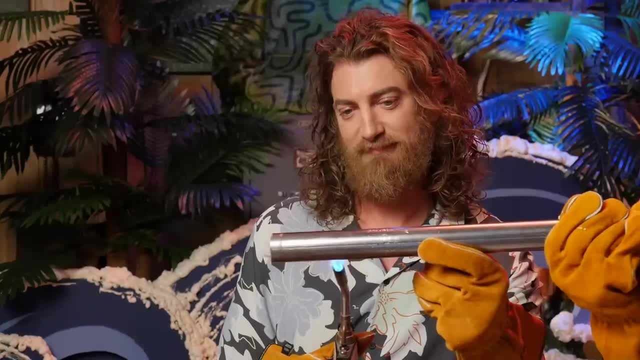 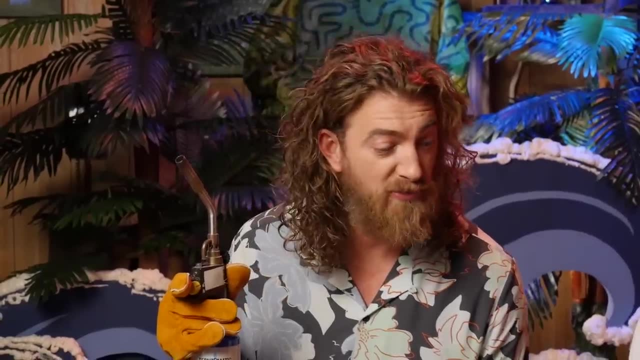 Was that you or the heat? It was me, It was you. Ooh, that stink. Okay, we have to get the scientific principle. We gotta get the thing from Stevie. We have to get the information. We know it's a sound. 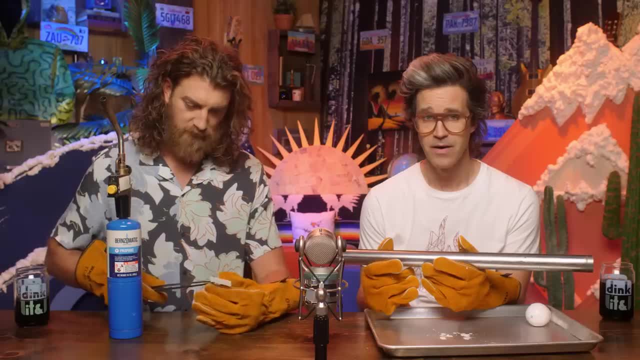 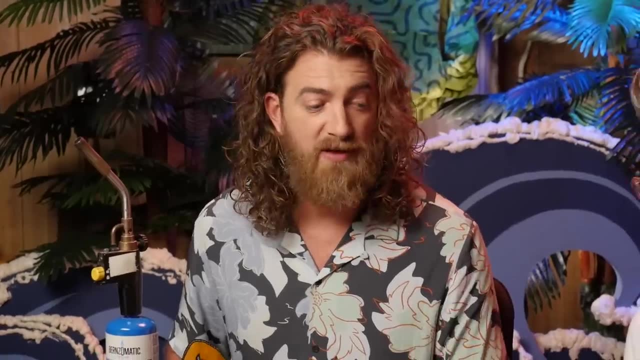 This result is so exciting it makes you want to break out in song. We didn't learn anything there And now we need. We know everything we need. You tell us a little story. Which end is the hot end? now I think that end yeah. 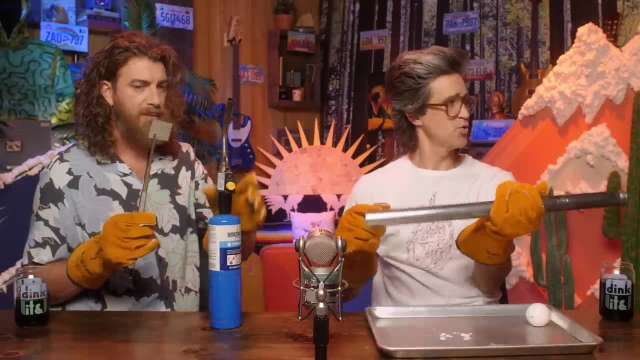 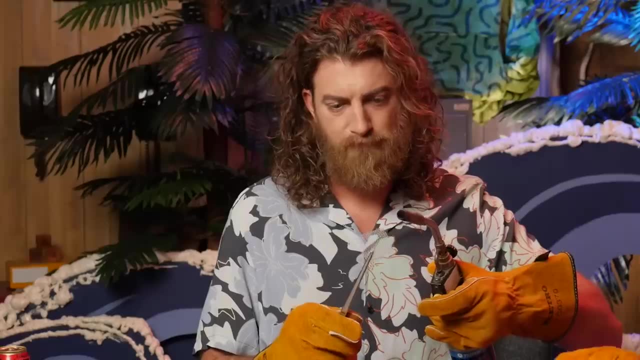 You tell us a little story. I'm not gonna get this. Is this in the hot end, Are you sure? Because I'm about to put my mouth on it? Bling. you tell us a story Gonna heat this screen up. 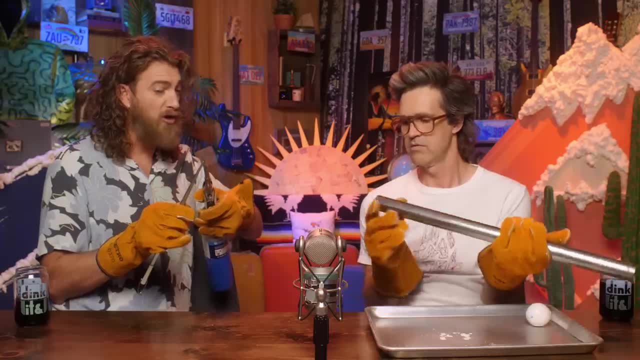 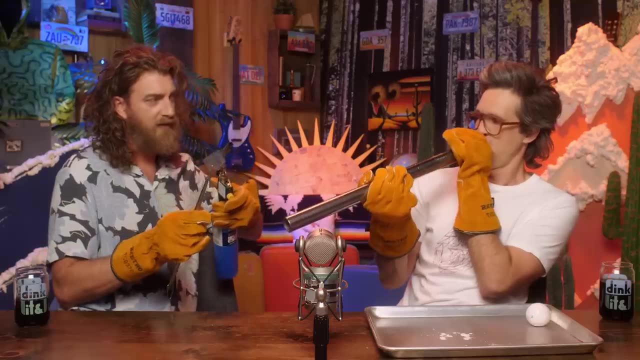 Whoa, look at that, It's boiling. You tell a story through the tube. Well, I don't know which end is hot. You think everything is hot, man, But there's heat coming out. There's heat coming out, yeah. 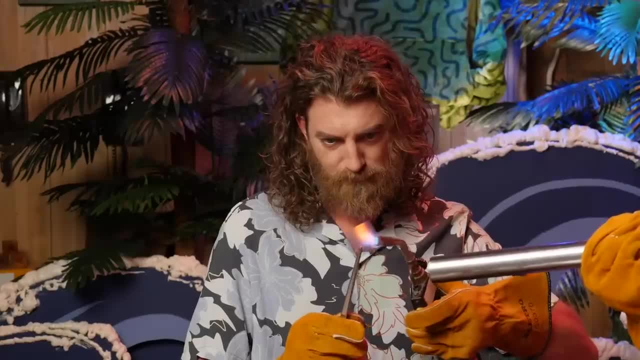 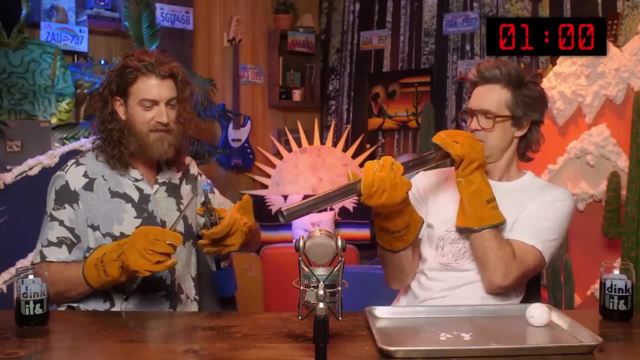 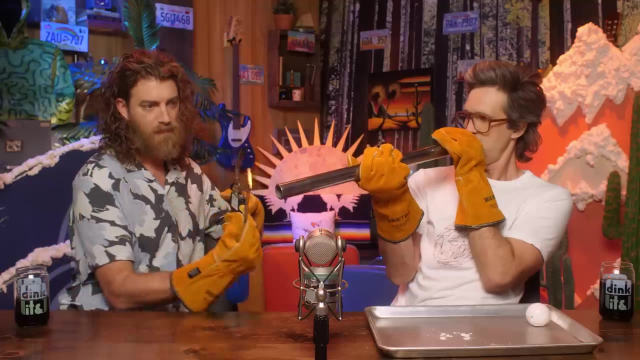 Now tell a story. Once upon a time you were using the blue torch. Hello, Don't change it. when I put it up there One minute, Make one note. It did something. It made a noise. I blew it out. 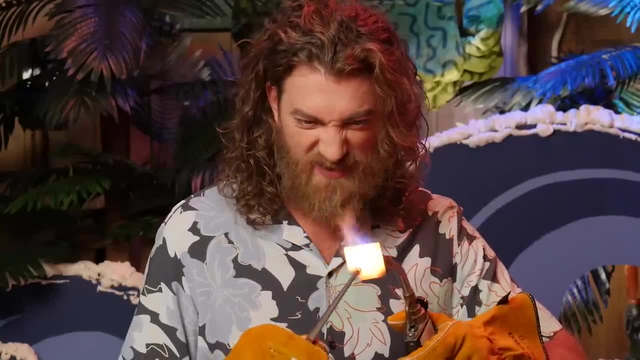 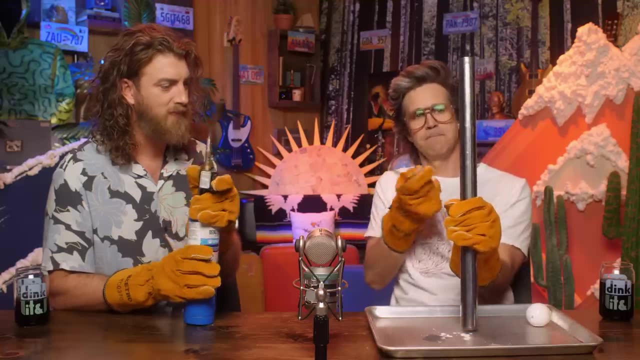 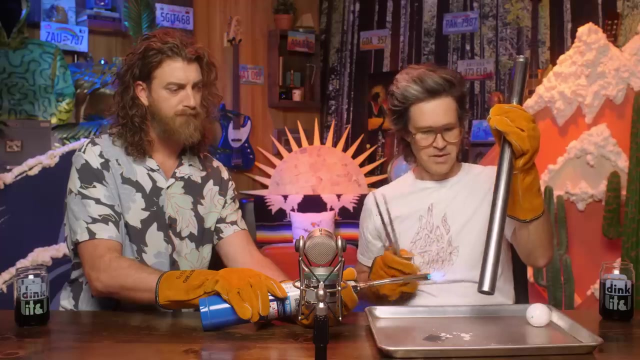 And it is not. a whole lot of hotness is coming out of it. Look at that, That's crazy. Now heat it up. God, It's not turning off. We suck. We're failing man, We suck man. 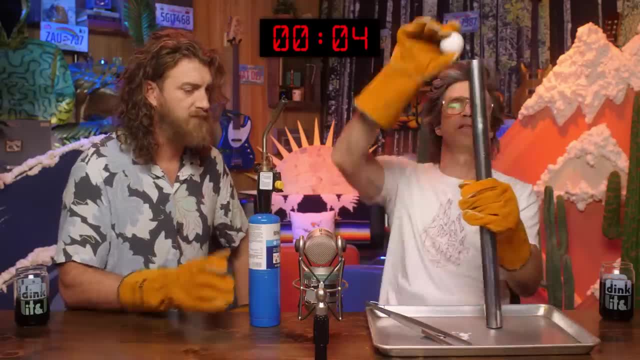 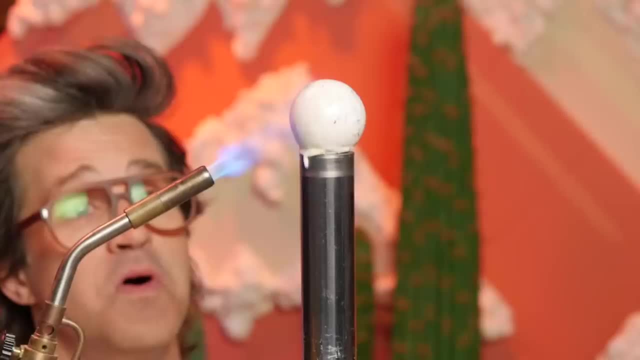 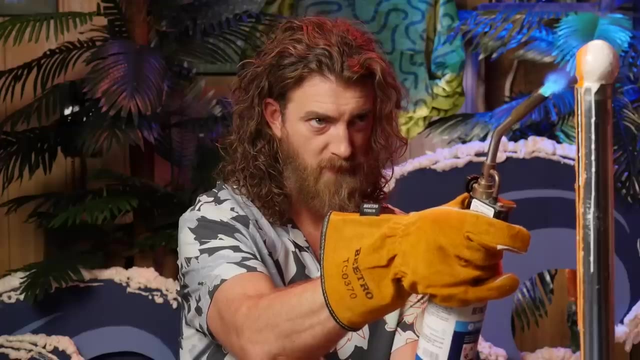 We're failing. I know we were on the right track. You know what? Let's just melt this completely. It was cool. The best thing we did was that And time. Look at that. Eventually he's gonna fall in the tube. 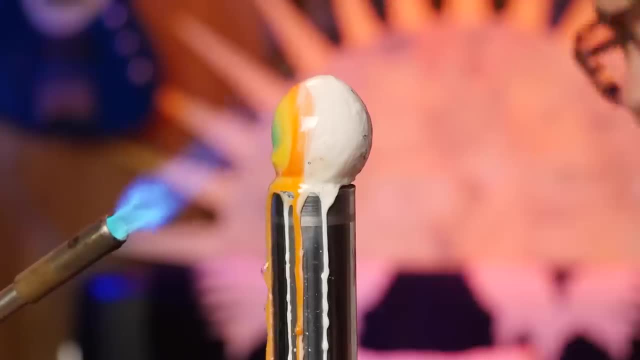 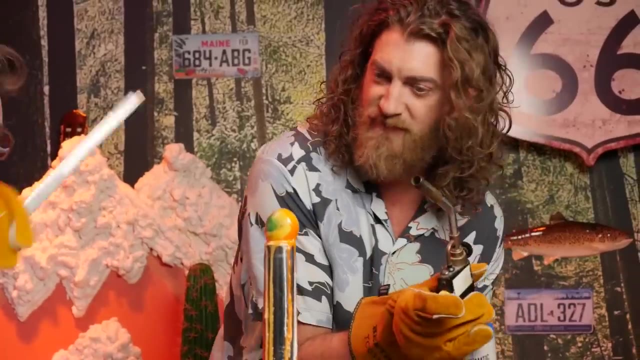 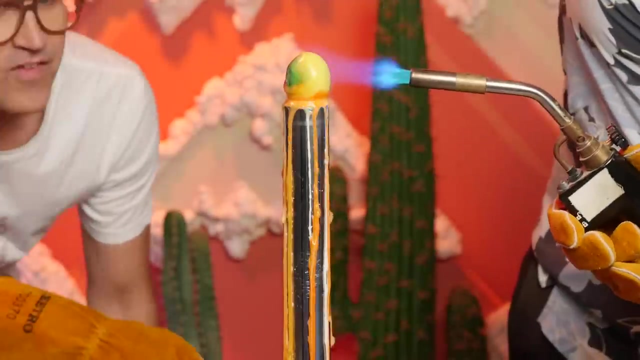 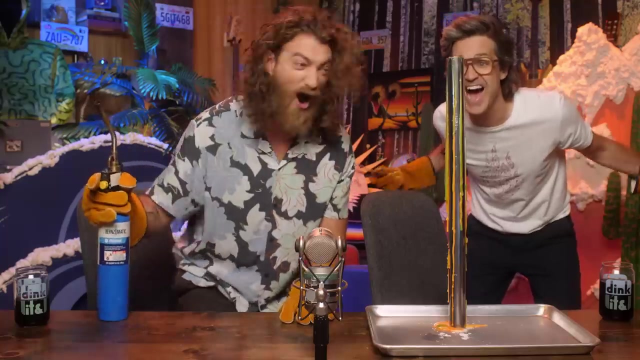 when he gets so small. We could go down to Venice, man, and just put a hat out. people would start putting money in it. Here we go. Whoa Yeah, Thank you, the hat's coming around. thank you, thank you, thank you. 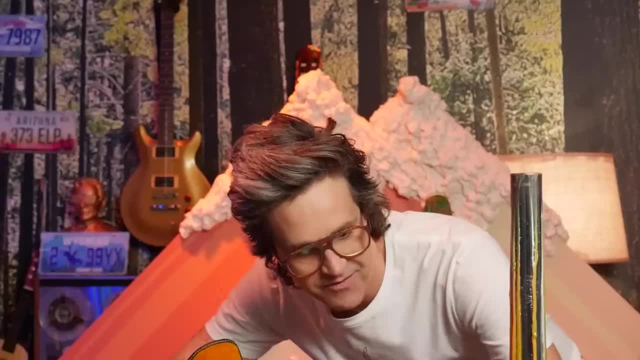 we'll be here tomorrow at the same time. thank you, thank you, thank you. And then, if I pick this up, Oh, oh, oh, you made art man, look at that. So, Stevie, we did it. 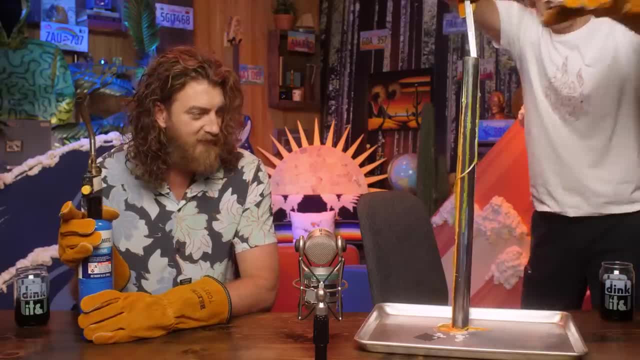 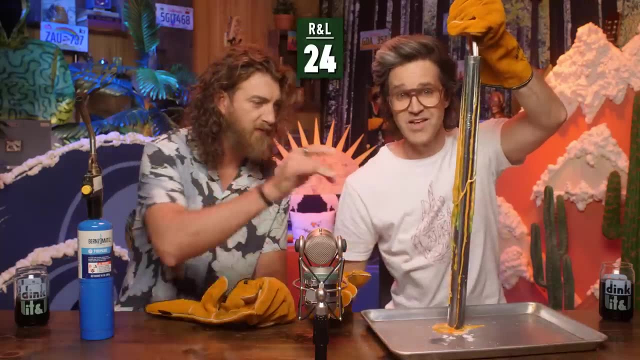 Yeah, yeah, we did it. what we're saying is: we did it. I mean, it is hard to believe, But that is not what we were looking for. Look how cool it is, though, But I will tell you who did get it. 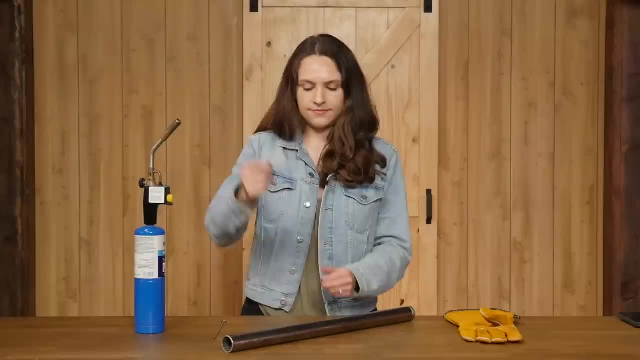 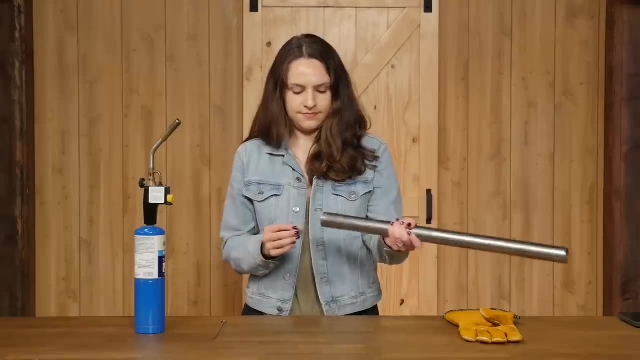 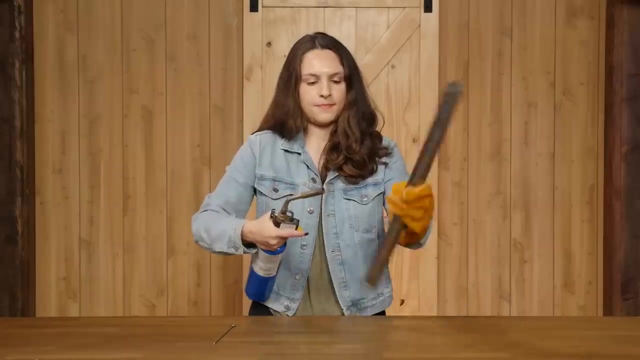 and that is Caitlin. Oh, so she did use that. Oh, and she folded it. I did that. look at that. you did that. Oh, I was on the right track. You were on the right track. Oh, she shoved it. 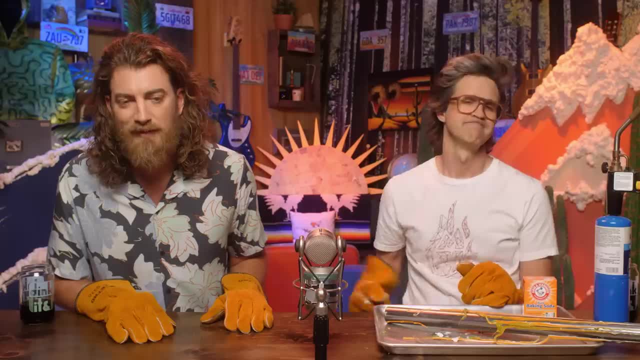 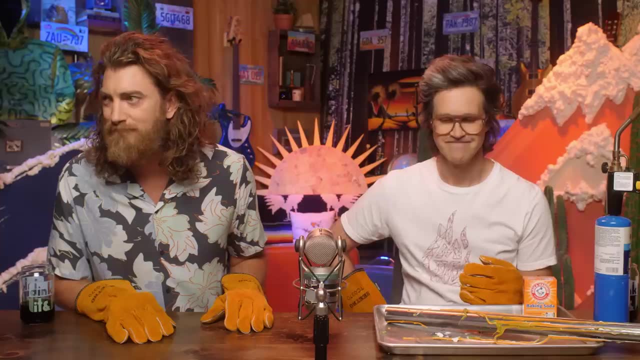 So it makes a reed. I was completely right, but I had no idea. So here's how it works. The blowtorch rapidly heats the heavy gauge metal screen inside of the pipe. as the hot air rises, cool air begins to be pulled up through the pipe. 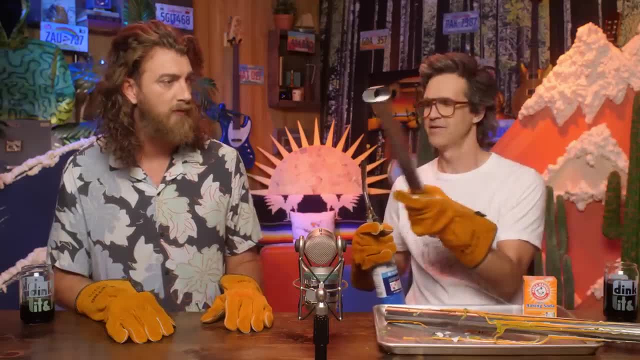 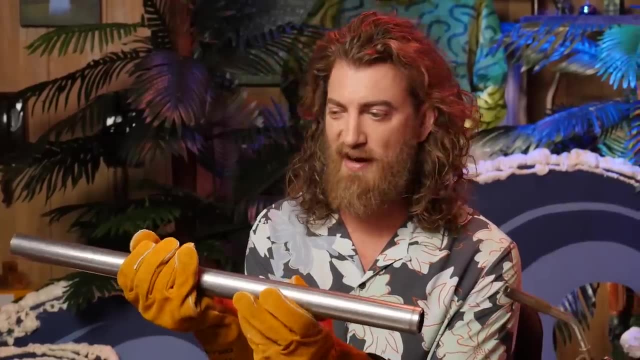 the air moving through the pipe vibrates the metal screen, which leads to resonance inside the pipe, causing the pipe to sing Like an organ, but like a really hot one. Here's one for us to try. Oh, that thing's hot, yeah. 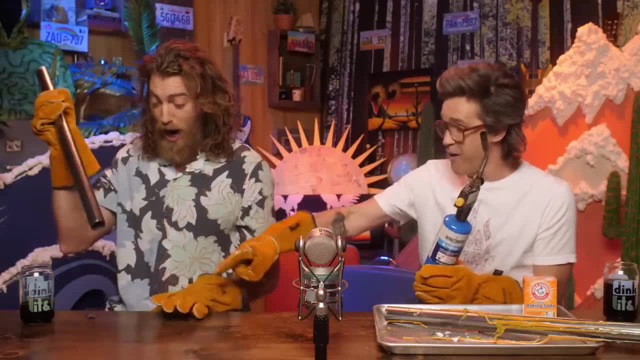 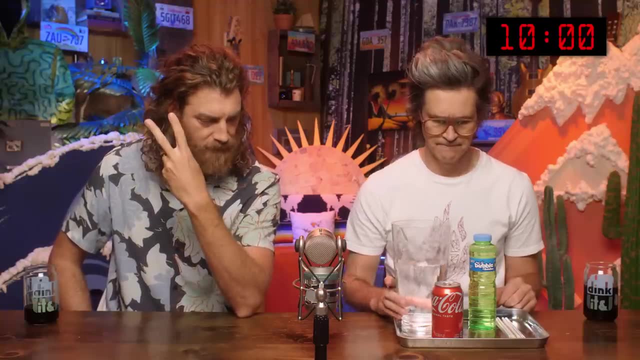 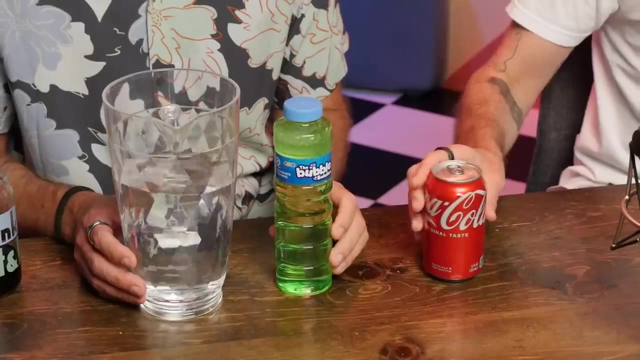 Okay, Oh, watch out, watch out, watch out. Your lifelines are the same. there are still two decoy items and your time starts now. We got some water, That's just to stay hydrated. We've got some bubbles. we've got a can of Coke. 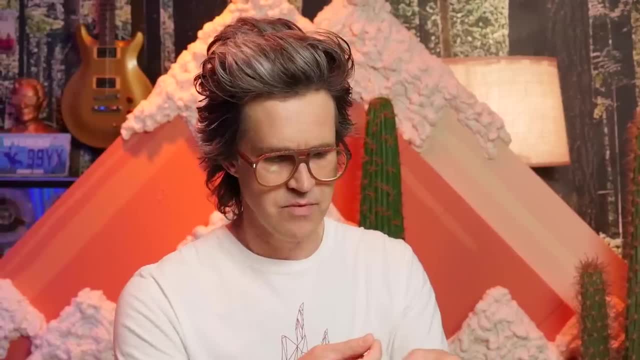 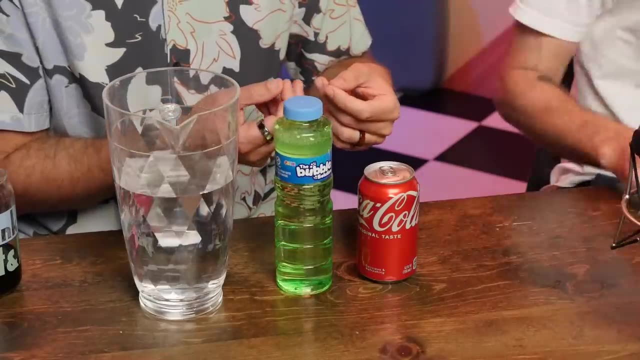 we've got string that's already tied, Tied in. what a loop, A loop. and then you can Well, that's a bubble, Maybe you can put. that's a bubble maker waiting to happen, try that. And then we have straws, four of them, four straws. 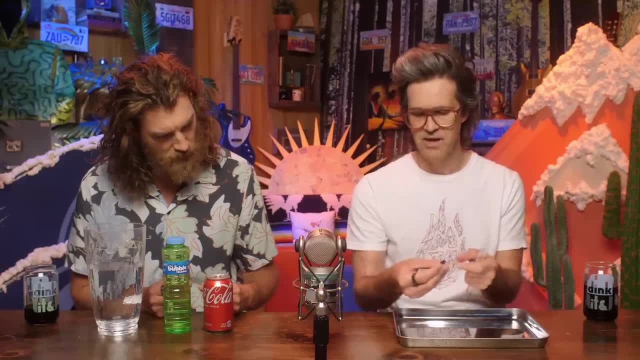 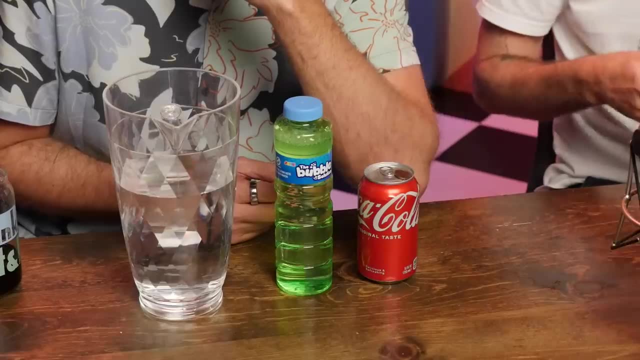 So I bet you we can. can you make a long straw with that? And then finally, we have a penny. This one has Lincoln on it. Penny feels like a thing that doesn't matter. Bubbles and straw- I mean pennies- don't even work the penny anymore. 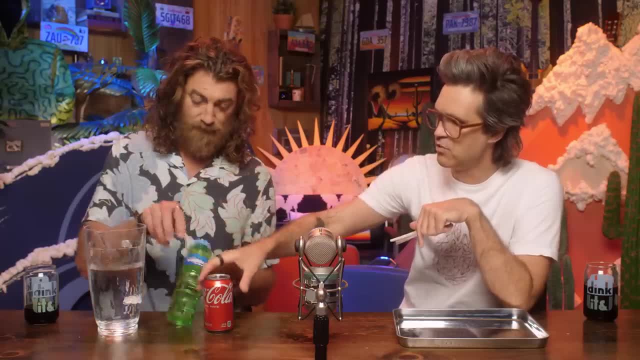 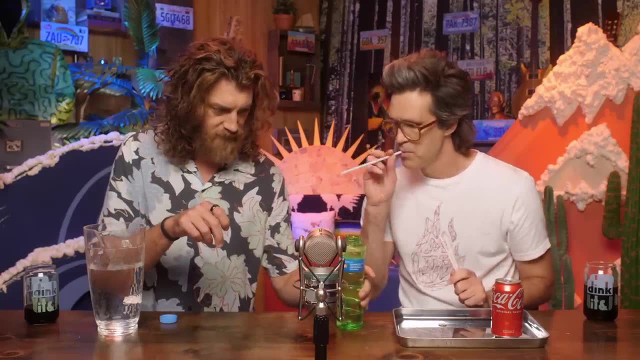 Try to even see if you can make a bubble with the ring there. I mean, I have to think you can Here pour some of this in the tray. Well, the tray's not part of it, so we can't. oh, you're just saying to get rid of it. 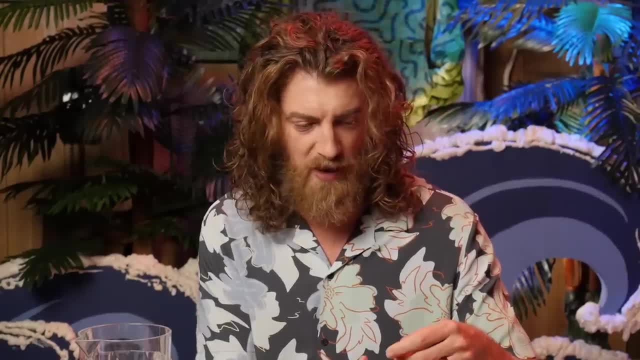 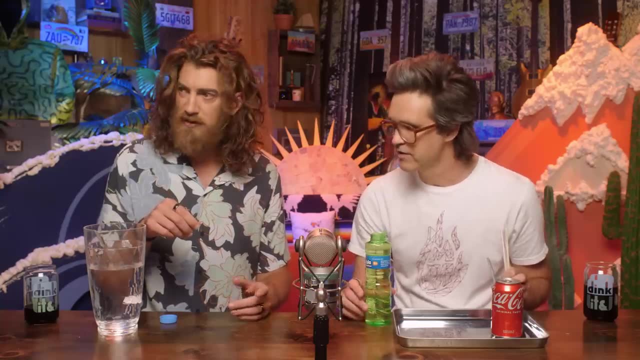 No, no, so I can dip it because I can't get the whole thing wet. Well then, but that's the wrong track then, because we can't use the tray for part of this experiment. Can we use the tray for part of the experiment? 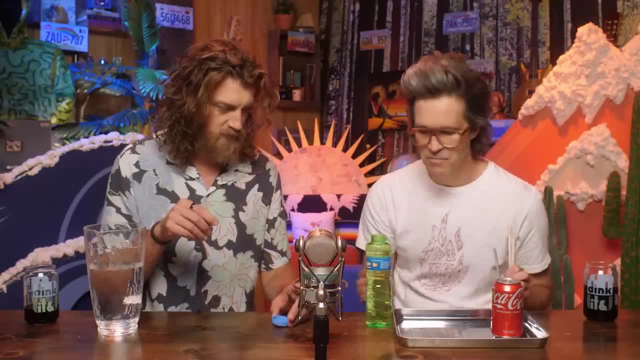 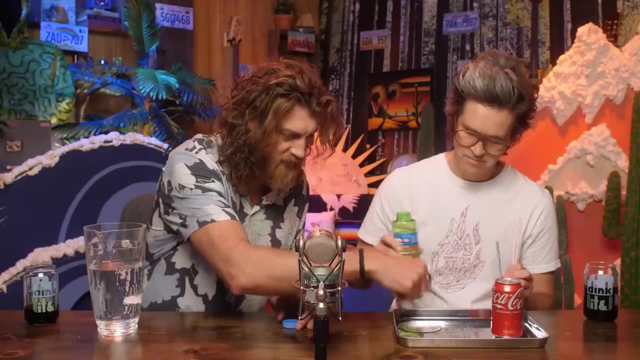 You may, Yeah, Well, you can't. I'm saying, of course we can, but we shouldn't, because the tray's always here, Yeah, but the tray's always there, All right, fine. So I'm just saying this is the way. 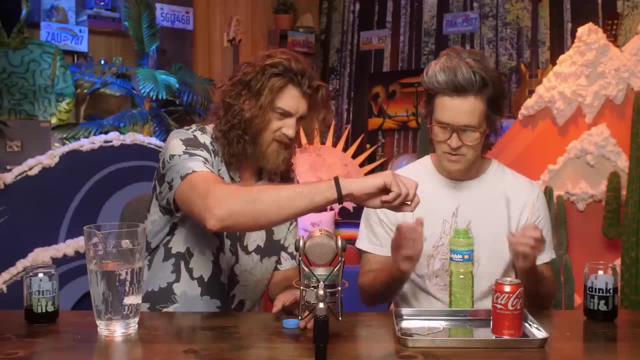 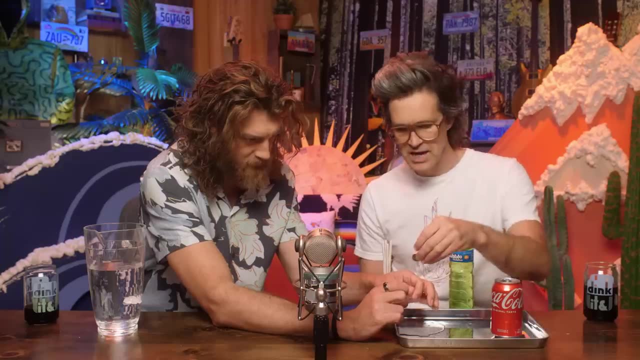 that I can actually get the thing completely wet And see, yeah, it's just like you gotta have like a Four straws in it. You gotta do something to get it. Then why would there be if you tied the penny to the-. 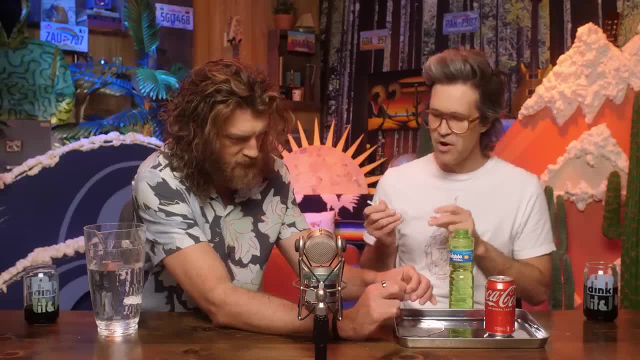 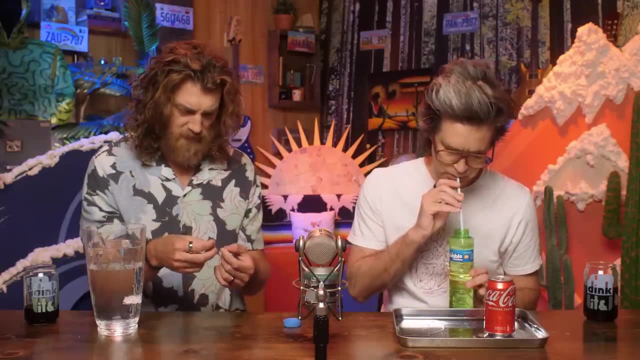 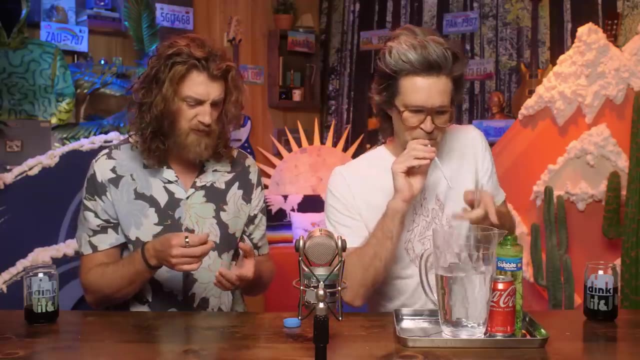 I don't think the penny's part of it, Like blowing a bubble under water, would be really cool. This is way too much dexterity. Way too much dexterity. I'm gonna suck up some of this Blowing a bubble under water. 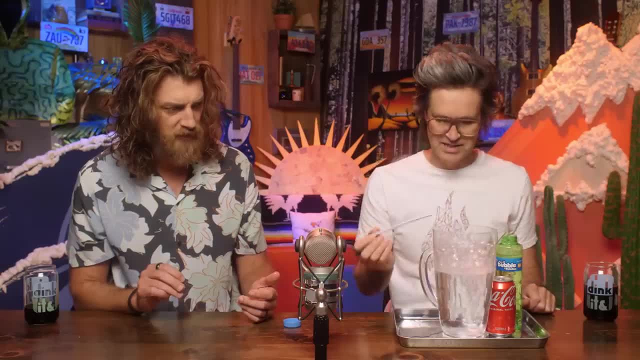 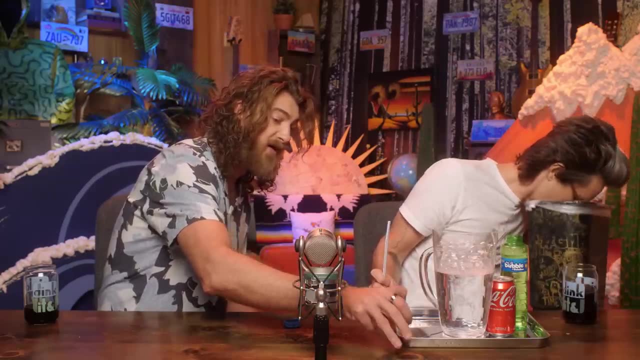 Yeah, it's just gonna be a bubble under water. Look at that. Yeah, All right, we did it. I think we got a lot. Actually, we got more. We got what we needed from Makayla's hint last time. 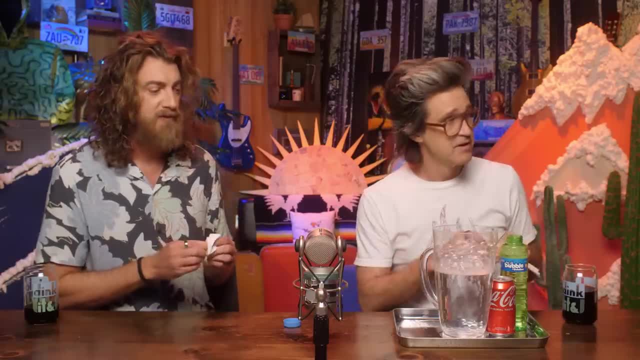 Yeah, and it's cheap. And it was a bit redundant, She's not cheap. So okay, Makayla, let's get that, because I think that helps us establish what's a decoy. God gosh, taste this. 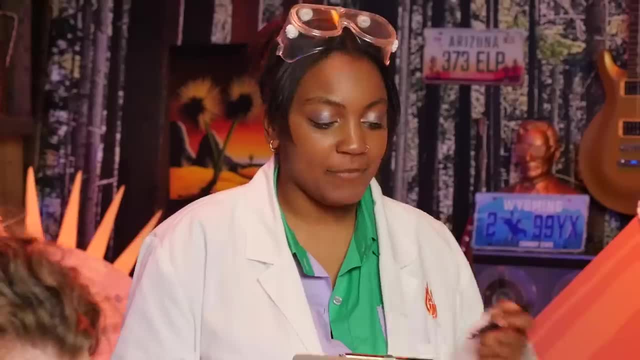 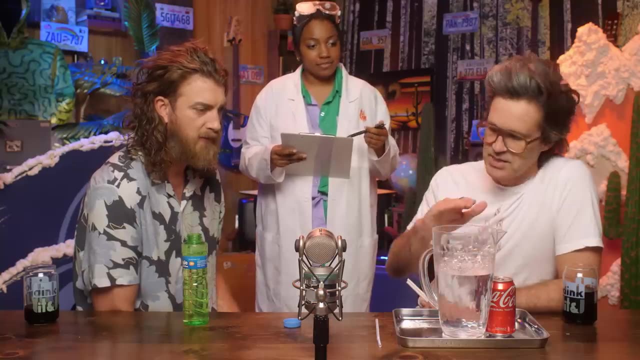 I just wanted you to know how bad it is. Yeah, I trust you. Okay, things can seem really tense on the surface, but that's not necessarily a bad thing. Tense on the surface. So surface tension is what we're dealing with. 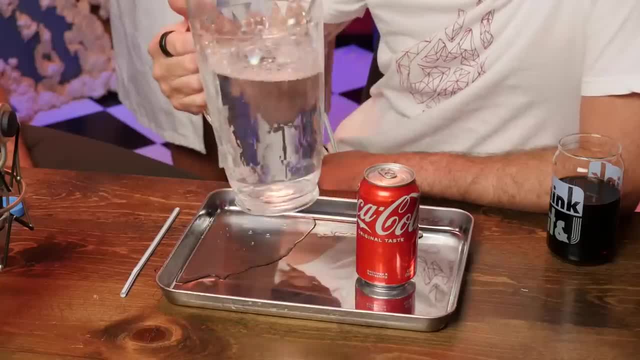 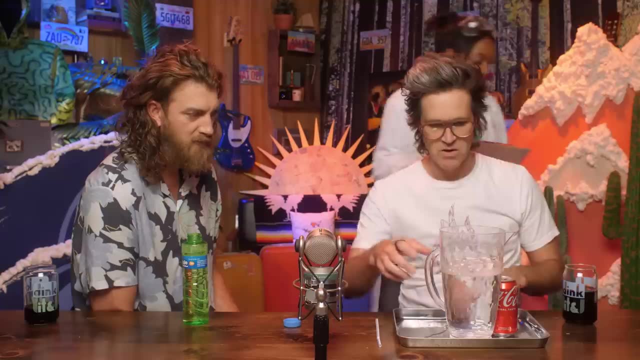 Surface tension. So we want to pour water, And now we've got bubbly water, which is probably a problem. We can get you a refill. We'll see. let's see. All right, I think we need another water. Oh, there's so much tension. 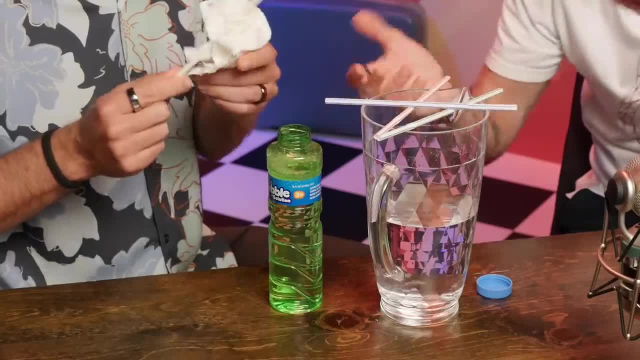 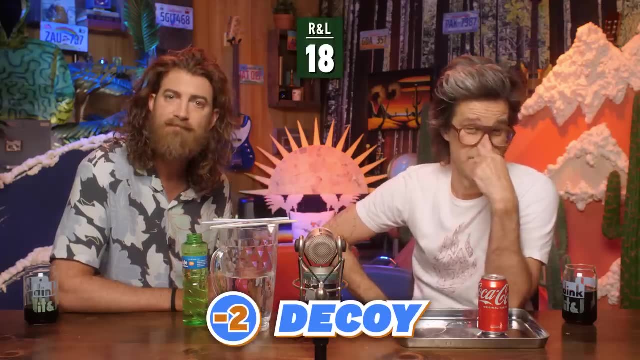 We can build a That's cool, I don't know. And then we did that one. I think we gotta get a decoy out. We gotta get a decoy out. Give us a decoy, You do not need the Coke. 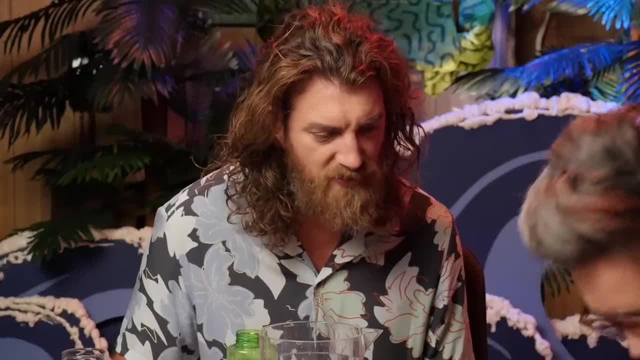 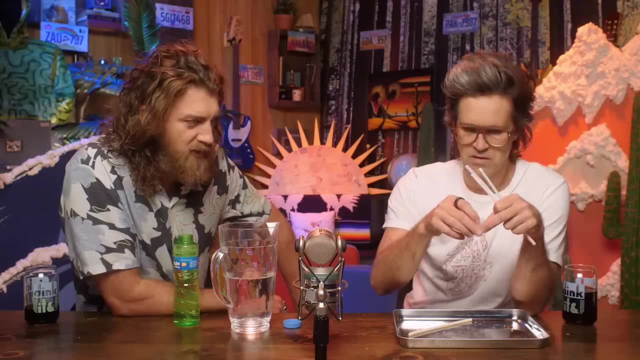 Yeah, Okay. What if you put the string inside the straw and then it like this is tough y'all. How do you do this? Can you tell us whether or not your hint is gonna be helpful or not, Because it wasn't last time. 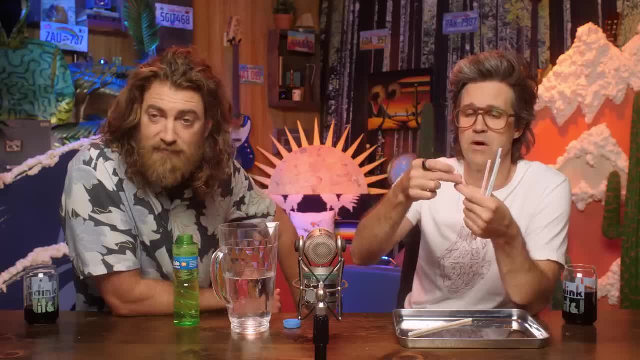 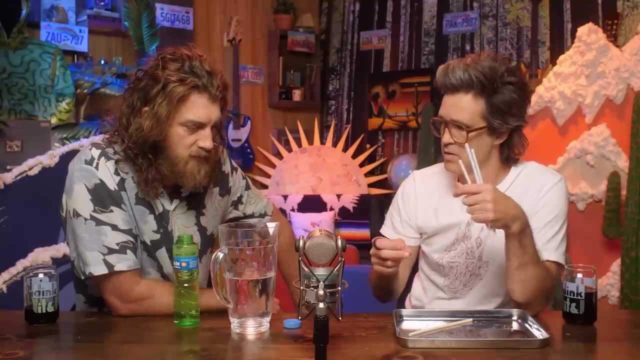 It is going to be helpful this time. actually, I feel like we gotta get it All right. we'll spend three points on it. Making a circle in a square is tricky, but not impossible. Making a circle in a circle. Making a circle in a square. 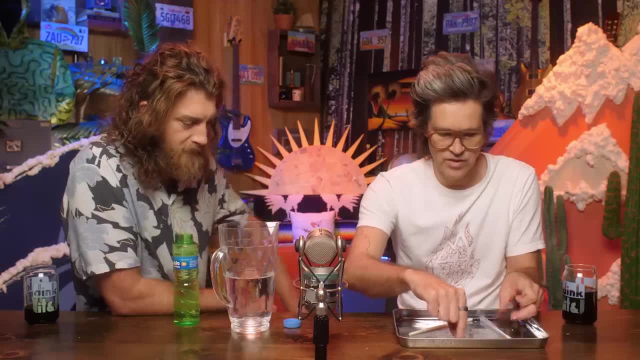 Making a circle in a square is tricky but not impossible. Making a circle in a square is tricky but not impossible. The only way to make a square is with the four straws. That's the only thing I know. We're trying to make a square bubble. 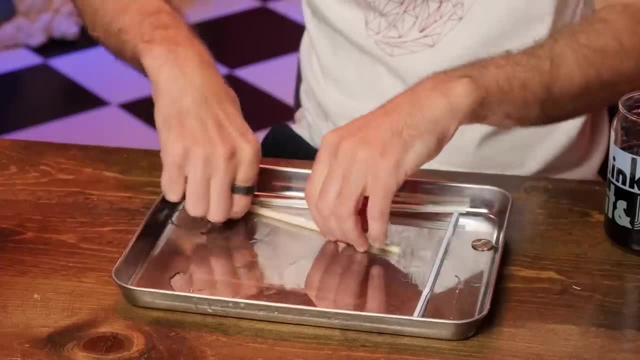 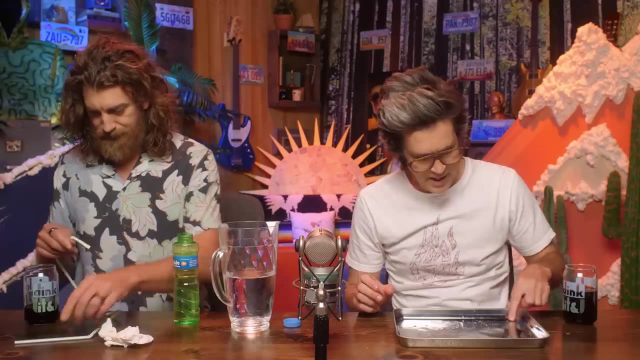 We're trying to make a cube bubble. Oh, you know what? These straws have joints, And then what you do is you can make a square. We're making a bubble wand, bro, And I don't think we need the penny. 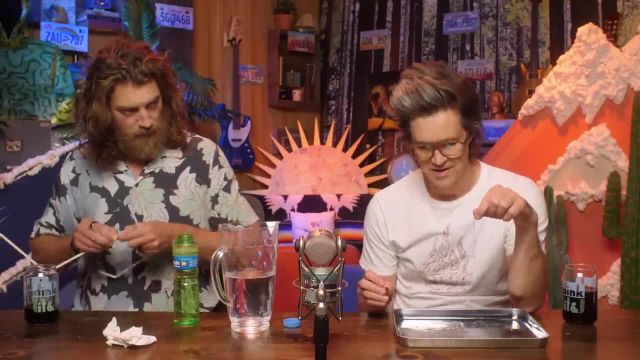 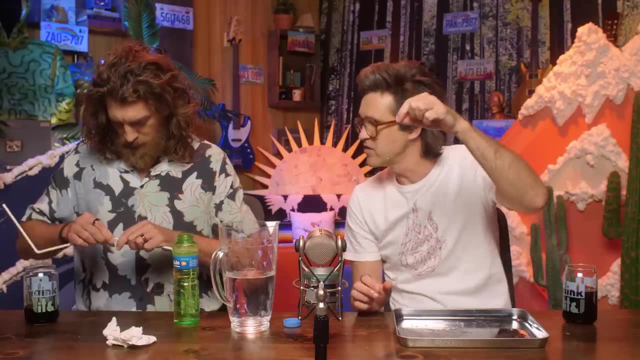 If we don't need the penny, then why do we need this? I think this here. put this around it before you connect it all together, so that we can hold it by this- That might be true- And pick it up And then blow it. 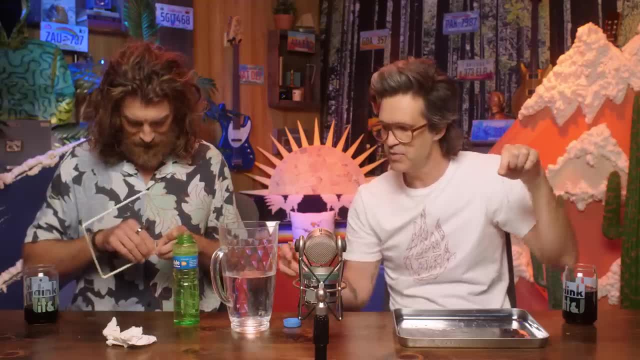 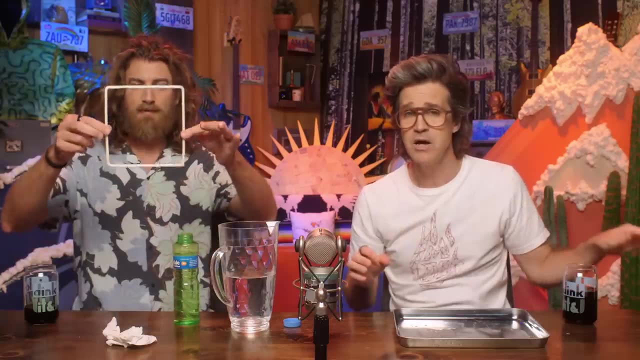 And then we don't need this. but if we don't need the penny, then we do need the water. What did she say? Making a square in a circle? Huh, Reverse. Oh, I didn't hear what she said. 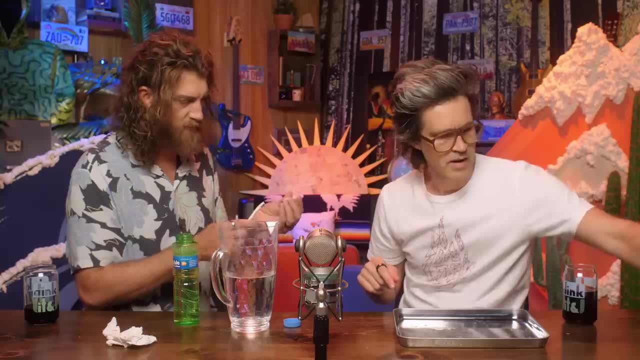 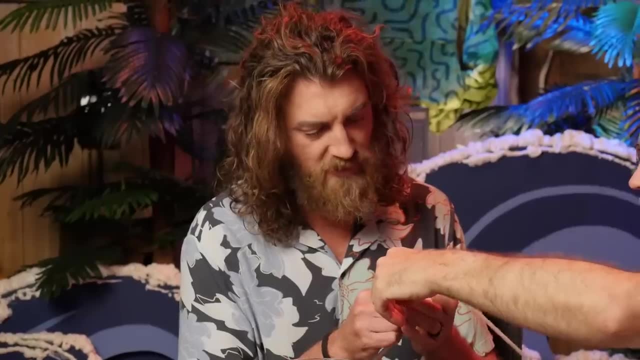 Making a circle in a square. Where's the thing, Where's the string? Right here? Put it on there, Right there. Making a circle in a square is, I think it's basically making a bubble with a square, And then we're gonna take this. 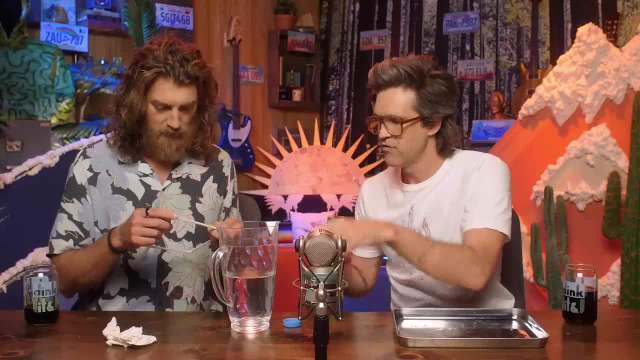 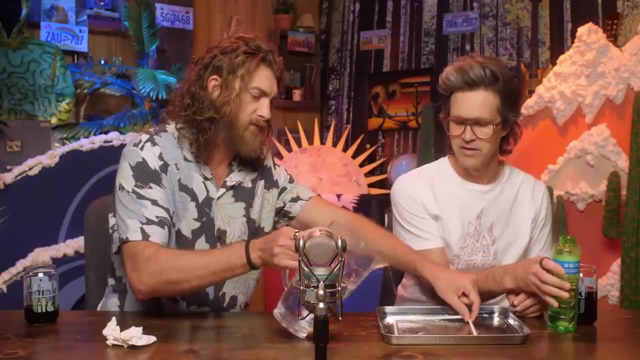 It's actually a dot. But then, Rhett, how do we use the penny if we're not using the water? If solution gets into eyes, rinse immediately with water. That's why we need the water. We just wanna mix it up a little bit, you know. 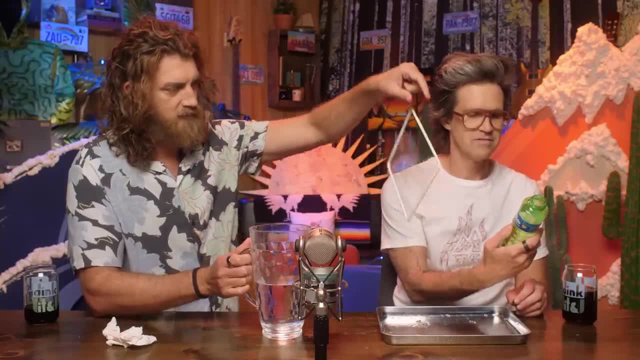 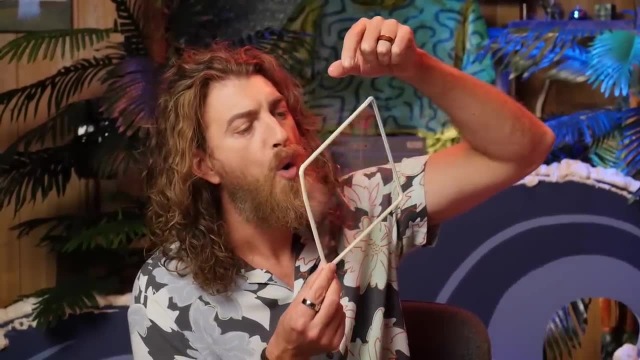 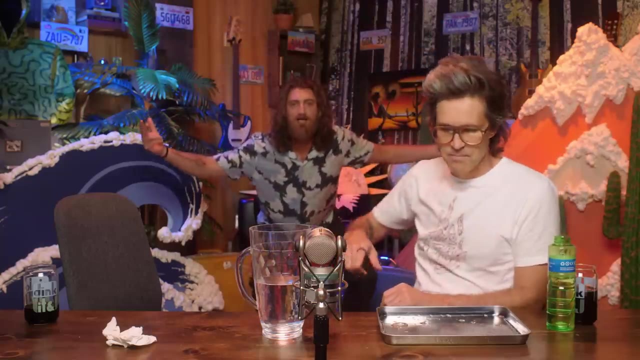 Since when you- this is not say concentrate, Look, see, look, there's a square bubble. Okay, and now? And I'm gonna blow it to the penny, Yes, that's a circle from a square. Made a circle from a square, jerks. 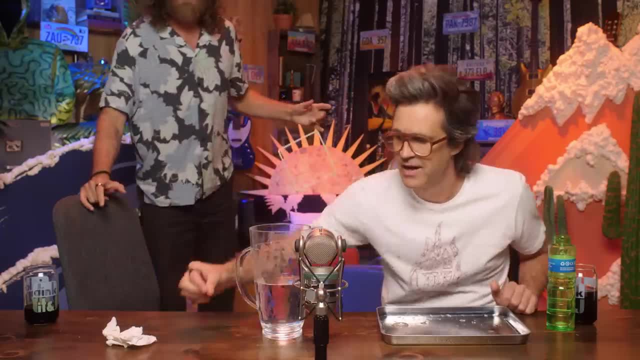 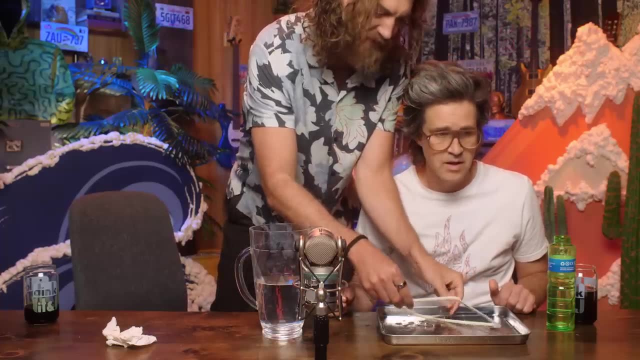 But we didn't use the penny. Yeah, that's our payment. I make a bubble, you give me a penny. One minute. I make a bubble, you give me a penny, Cause it's like again, we're back at Venice. 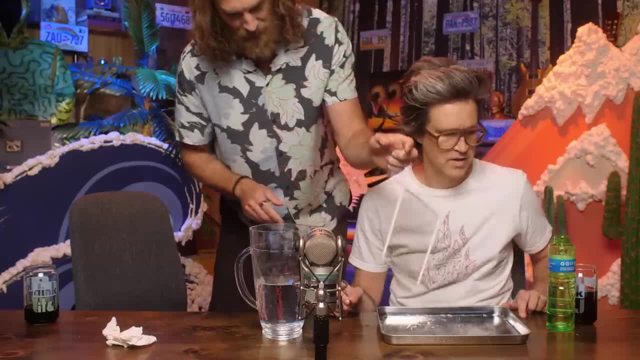 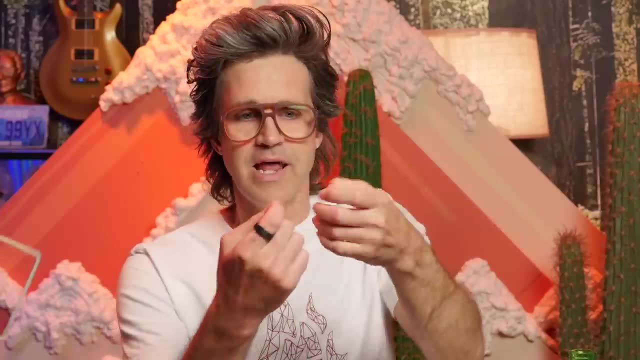 and all you got is a penny. 13 points remaining. All you got's a penny. What? All you got's a penny Give the man. Oh, oh, oh oh. look at this, Let's put this. make the bubble. 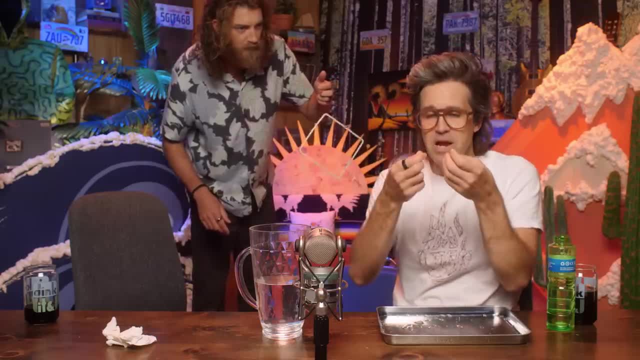 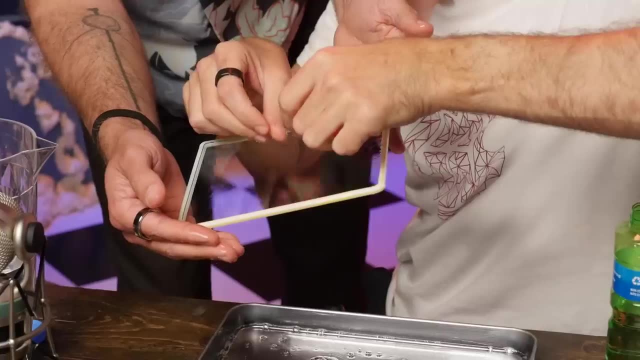 Let's put this: make the bubble. Let's put this: make the bubble. Put this on it and I'm gonna blow and it's gonna make. it's gonna make the thing through What It's gonna. Oh, oh, you broke it. 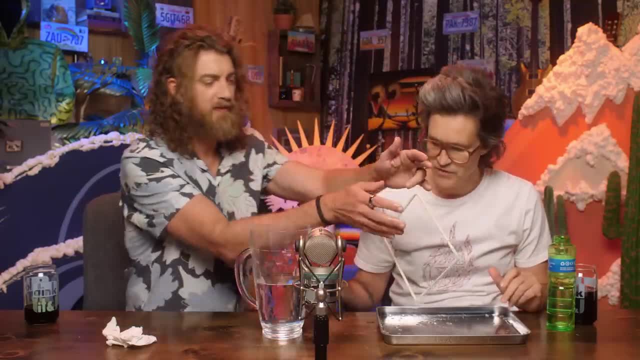 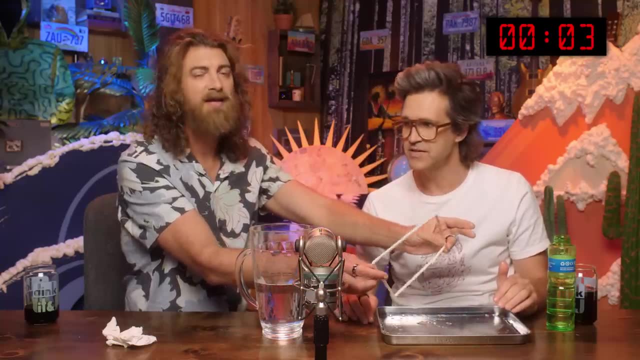 Okay, for two points. we can remove something. I gotta know if it's the penny or the. We got seven seconds. See, she gave me another one of these. I think we did it. Seven seconds, I just think we did it. 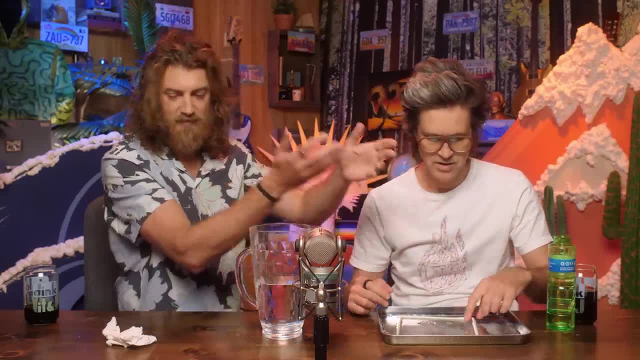 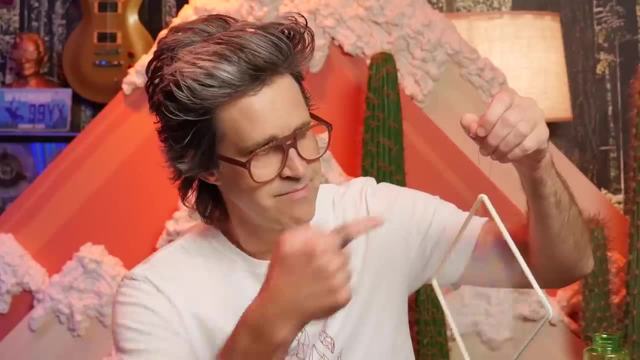 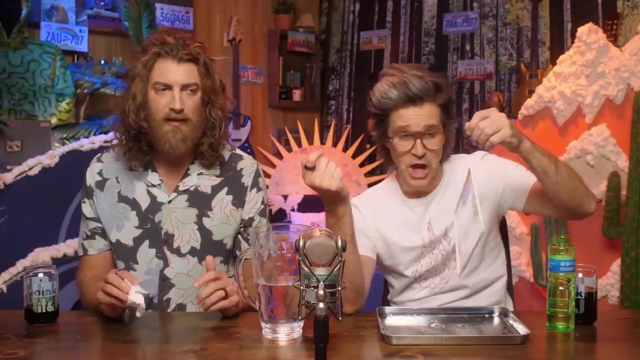 You're so close, your time is up, but I want you to get it because you're your instinct was correct, but you put the string on at the wrong time. What are you talking about? Okay, Caitlin, I'll bet you, Caitlin. 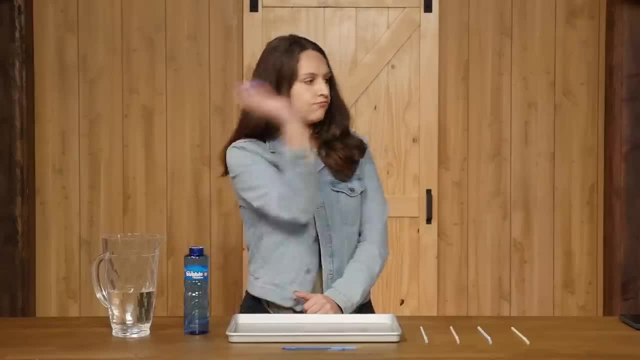 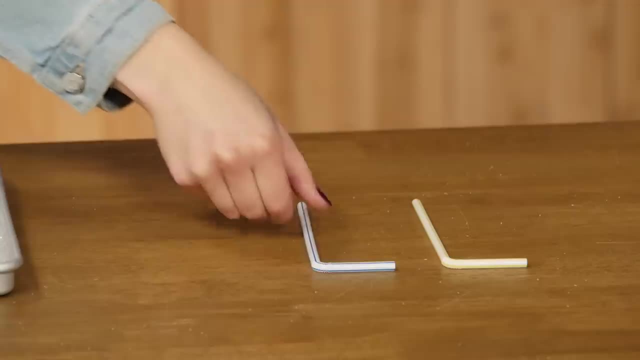 knows how to do it. Yeah, let's toss to Caitlin. She did use the tray. I stand corrected. She did use the water And the water, So I stand doubly corrected. But I did come up with a square. You did, you did, Yeah, you did. 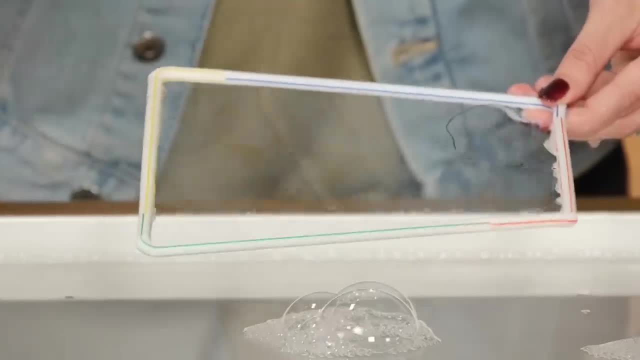 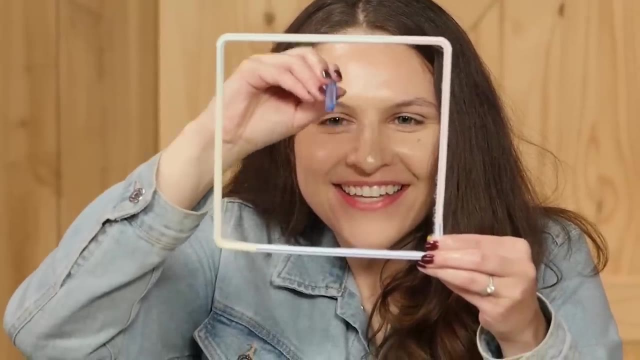 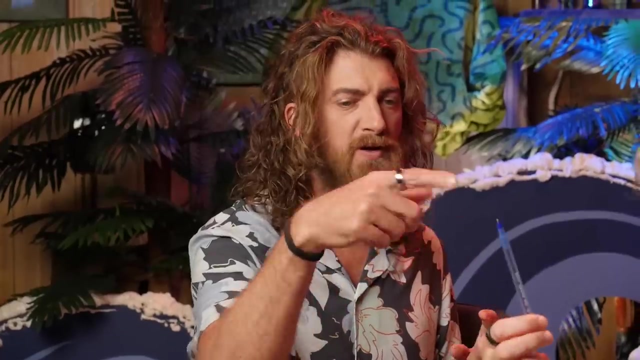 You did See, and I was trying to do that. Oh my gosh, Oh my gosh, We have to do it. Link, We have to do it now, But hold on The pen. the pen was not part of it. 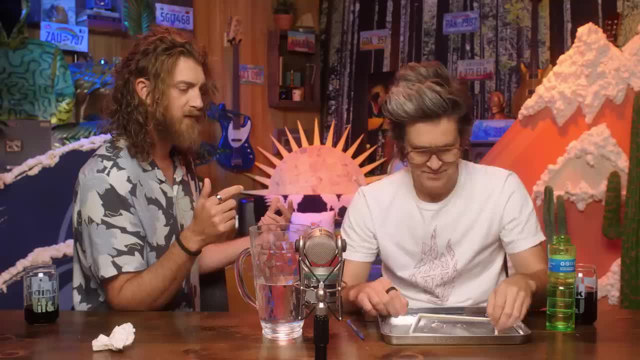 It could be your finger. It could be your finger, I'll do it with my finger. So the science behind what you're gonna attempt now is when you place a loop of string on a plane of soap and pop the inside of the circle. 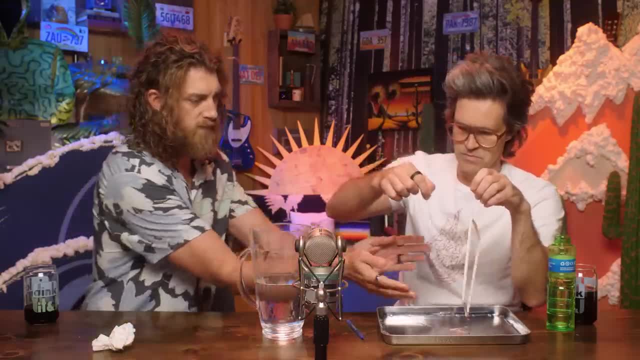 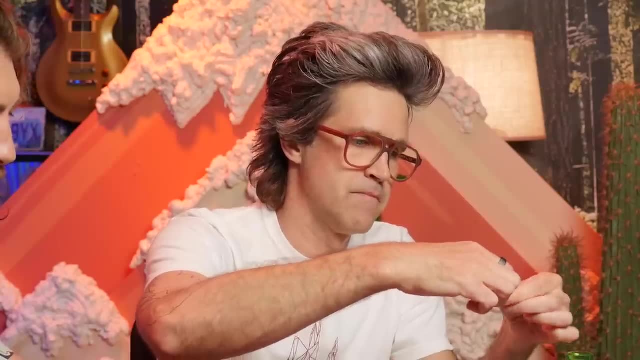 the surface tension of the soap pulls at the edges of the string until the string is, until the string has nowhere else to go. Once it's pulled taut, it forms a perfect circle. So all you gotta do is just get it on there. 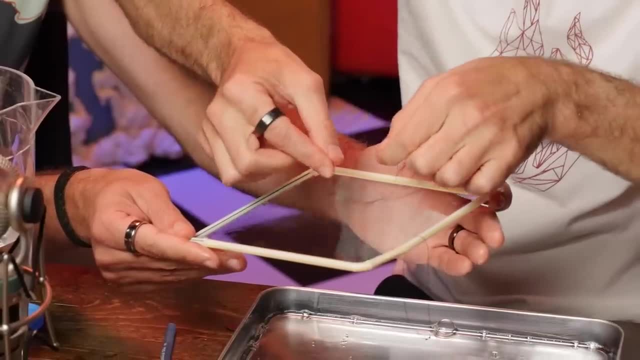 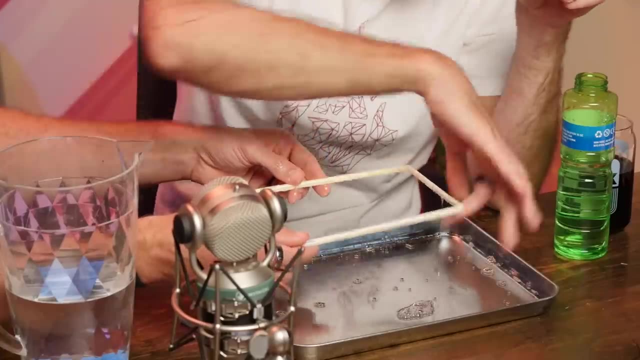 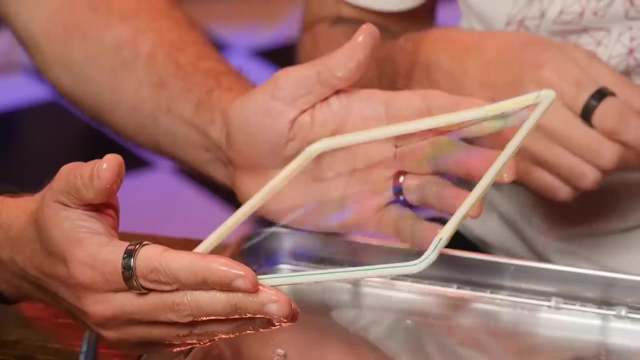 without it folding over Right, Which I can totally do like. oh snaps, It's hard to pick up. Is there a bubble on that? Just use this, Use it, we have it. Oh, there we go. Oh, you got the string on it. 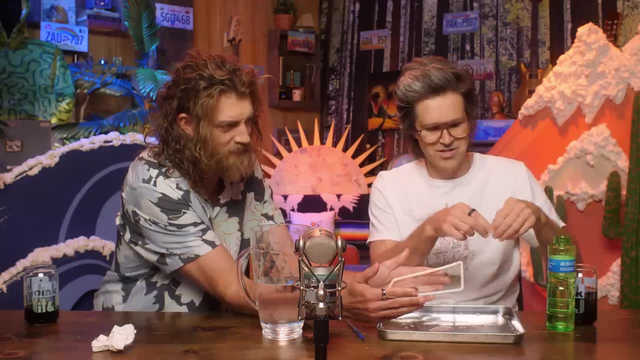 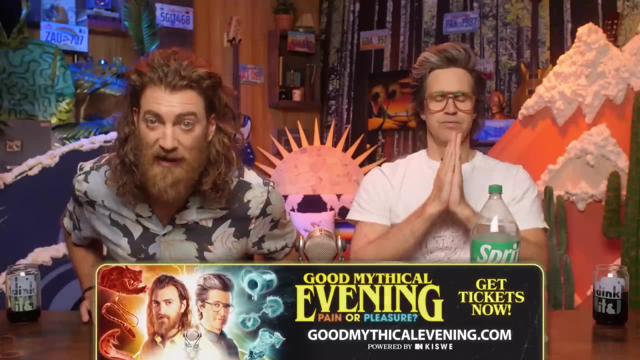 The extra string is leaning on it. I think that's okay. And then this string. oh gosh, I feel like such a failure. It pops Reminder Good. Mythical Evening is coming out real fast. It's gonna get wild, it's gonna get crazy. 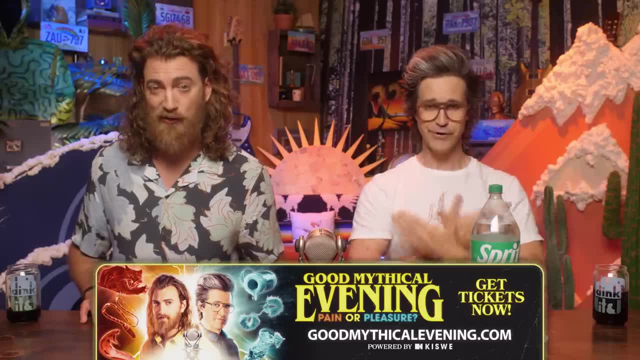 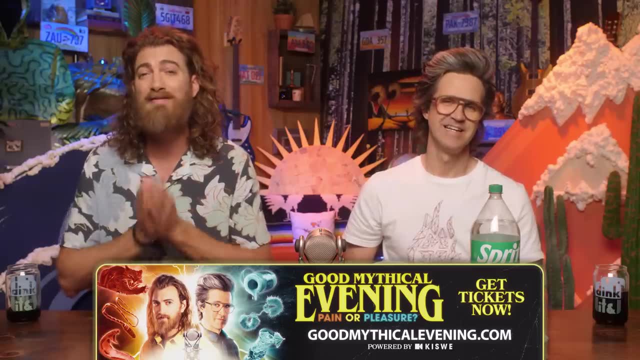 It's gonna be unhinged. We're gonna be plastered, Drunk and crunk. We're going live on August 24th at 10 pm Eastern, 7 pm Pacific. Tickets available now at goodmythicaleveningcom. 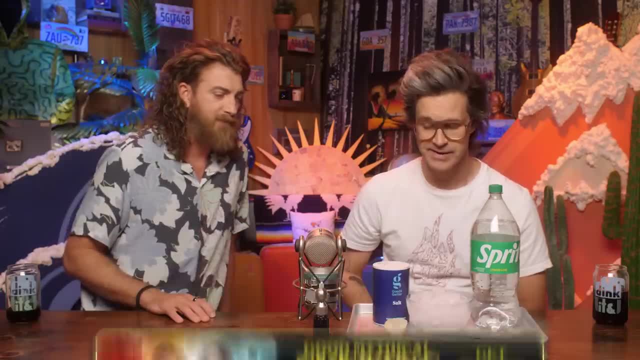 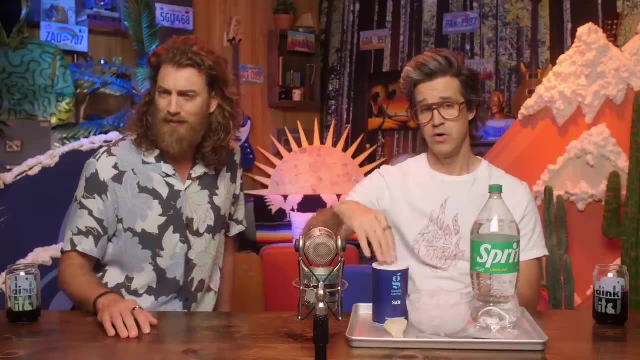 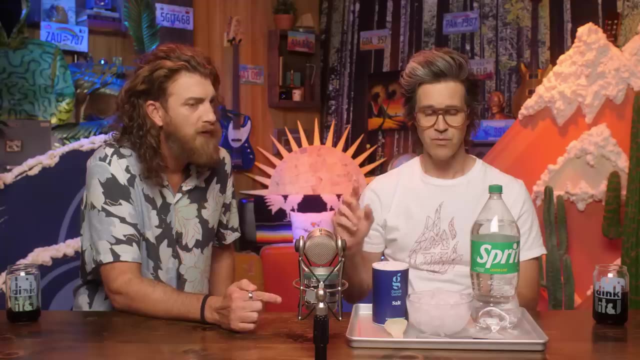 If you dare, Rated R, baby. Okay, so you have three decoys in this Round. We don't gotta do that. Same lifelines, Why Your time starts now. Link. let me make an observation: If we get Stevie, that's three. 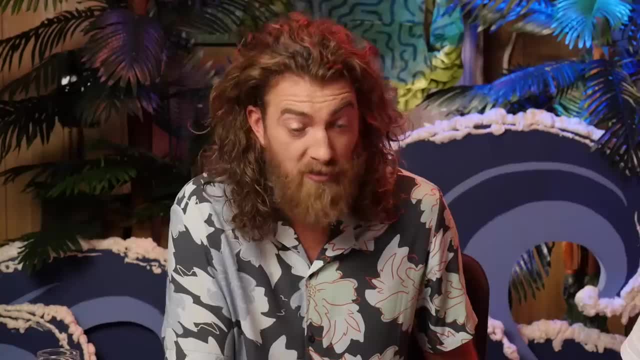 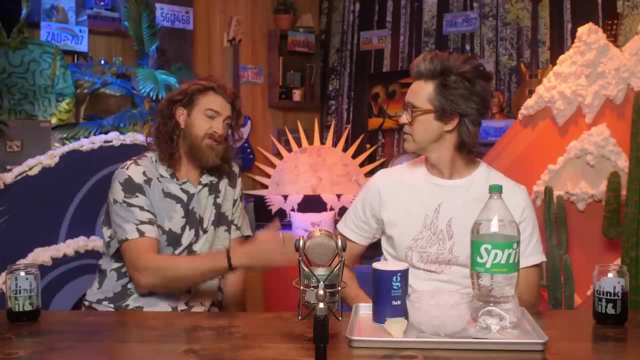 we can remove two decoys and still have a point and win. Well, that's a great observation. My observation was gonna be: we could just sit here and just chat it up, not even try, and we would just lose five points and still have three and win. 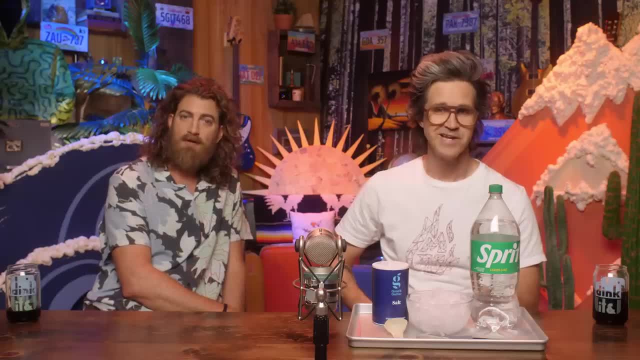 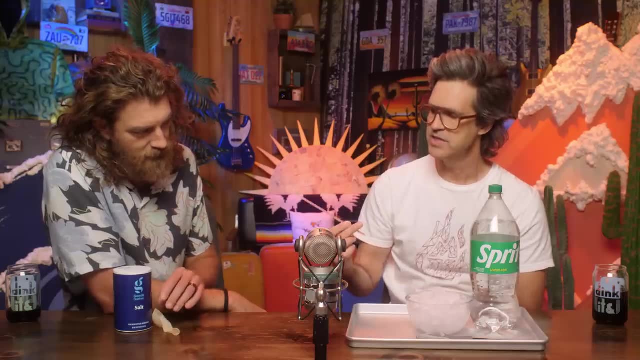 Yep, The Beaker Boys know how to make content, But the Beaker Boys wouldn't do that. Salt balloon glow stick. Yeah, Don't activate it yet. I've got an idea. So we've got a bowl of ice and we've got. 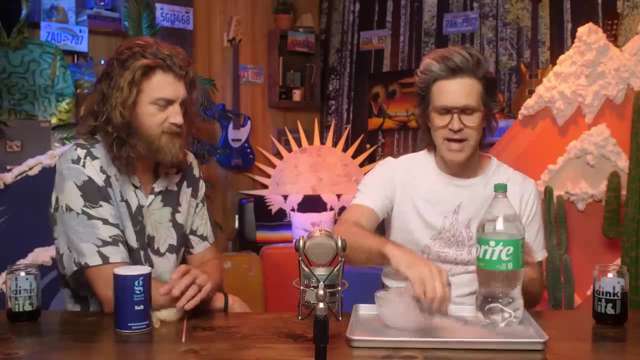 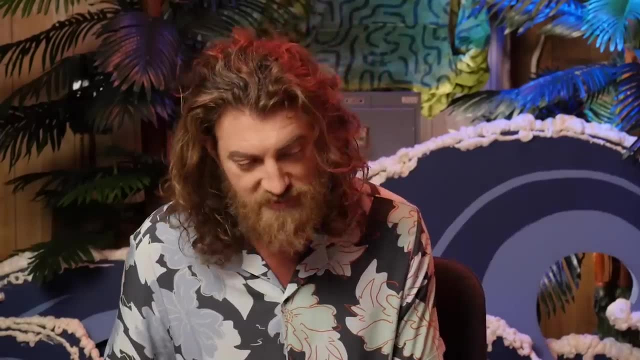 look-a-there, I found a Sprite. Sprite, I get it, And okay. Now, salt and ice creates a cold environment. So you're exactly what I'm thinking and I think that I think the Sprite I mean, if you put this: 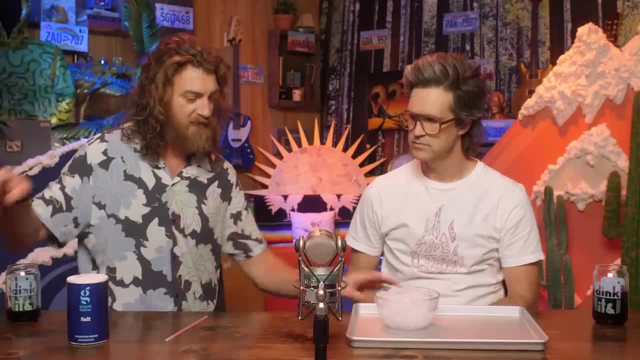 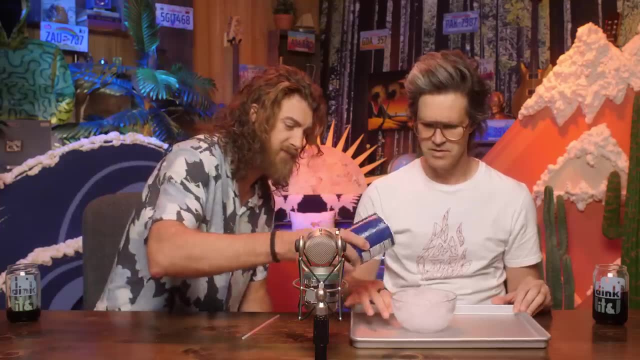 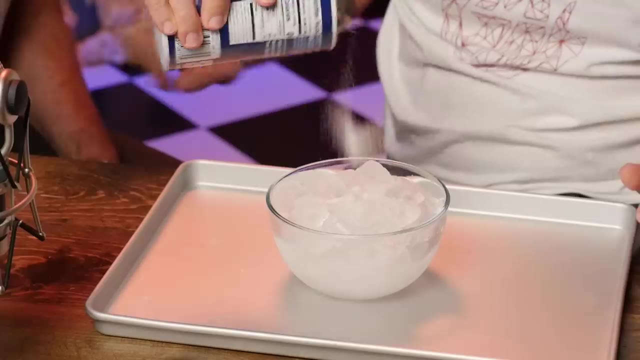 Decoy, I think the scissors Decoy, I think, the balloon Decoy, I think. just go with me here, I'm probably wrong. I bet you, if you make this super cold, something crazy happens, Okay, So this is like homemade ice cream. 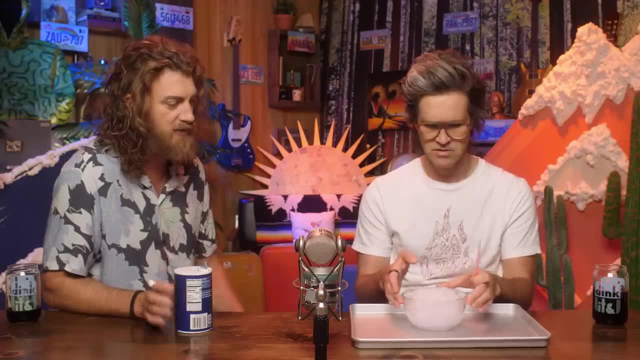 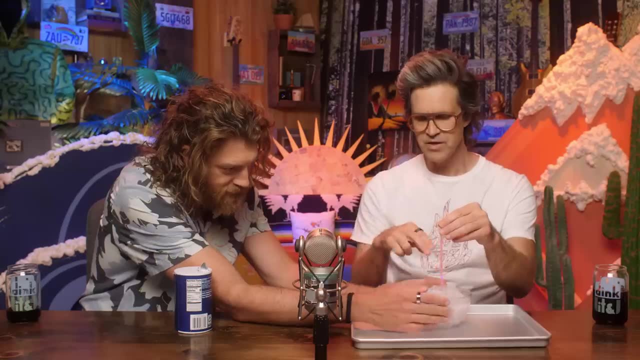 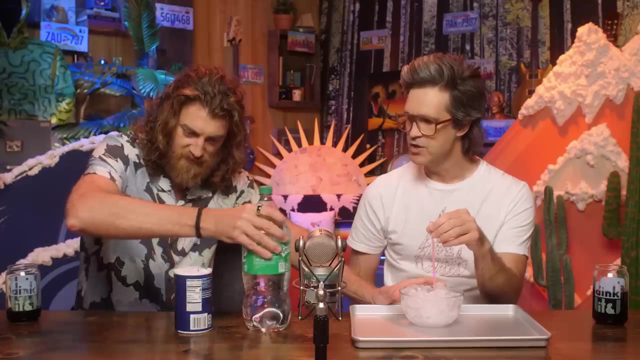 Mm-hmm, But typically it rotates. Yeah, you put it in there and I'll rotate. Okay, I think you should cut it and then drizzle all of the glow into something. But there's three decoys, And then you don't need the salt. 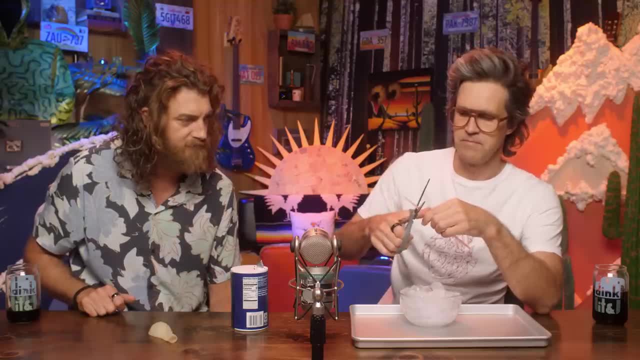 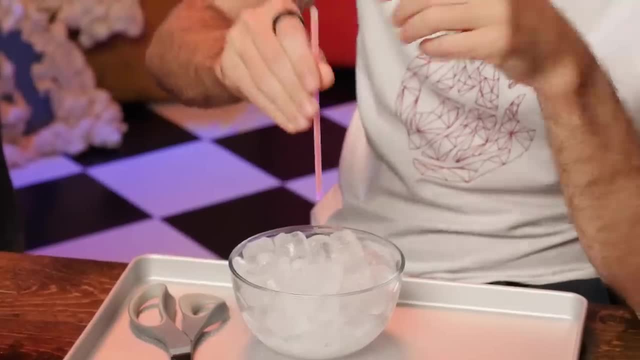 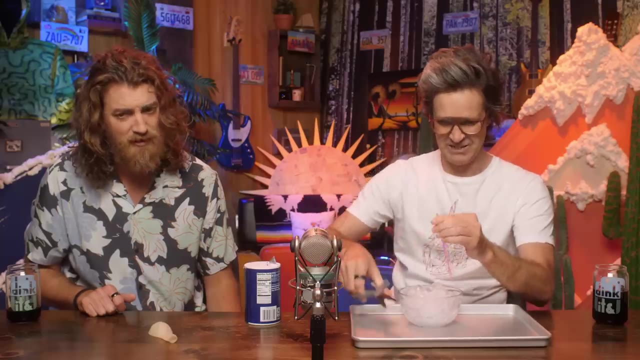 Carbonated beverages are always decoys. Isn't that poison? Stupid question. Yeah, All right. so do you Just put it on the ice? Oh, it's a gel. Maybe if I cut both ends and blow. Just don't suck. 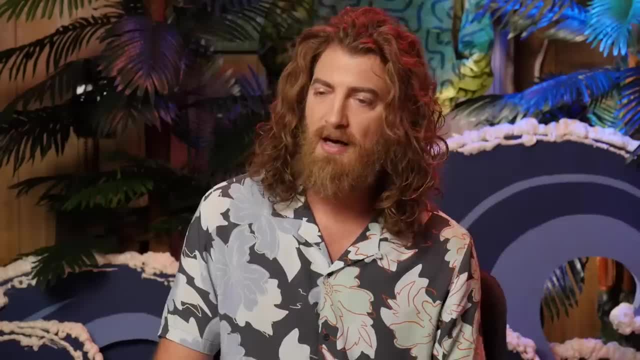 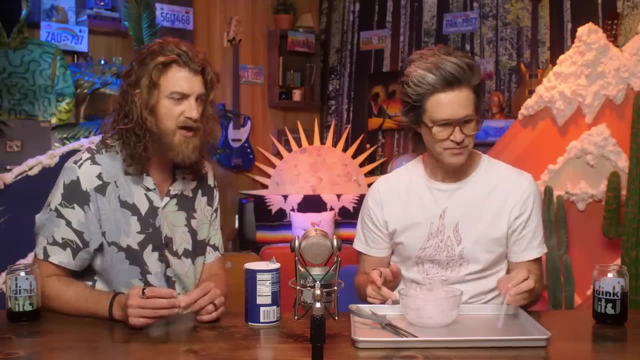 Okay, All right. so hold on. is something happening? New glow stick please? I feel like maybe That didn't work. Before we get, it's always more helpful to get the principle before you get the decoy. Yes, 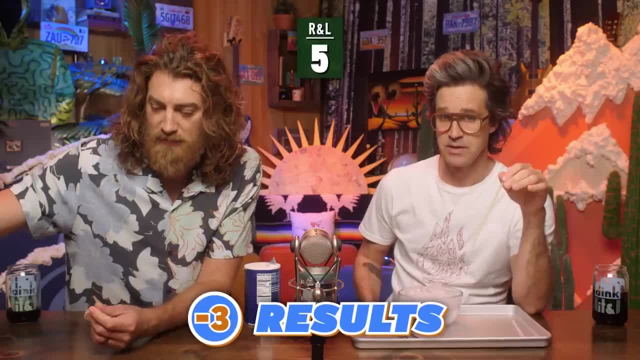 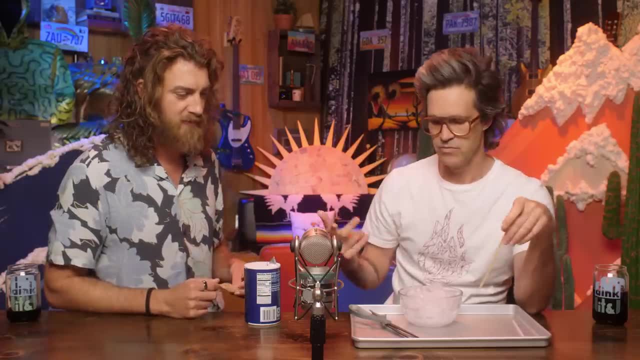 Stevie, what's up? Three points. You're looking for a way to inflate the balloon without blowing it up yourself. Well, let's just shake a Sprite and put a balloon on it. Okay, And we need to get rid of three other things. 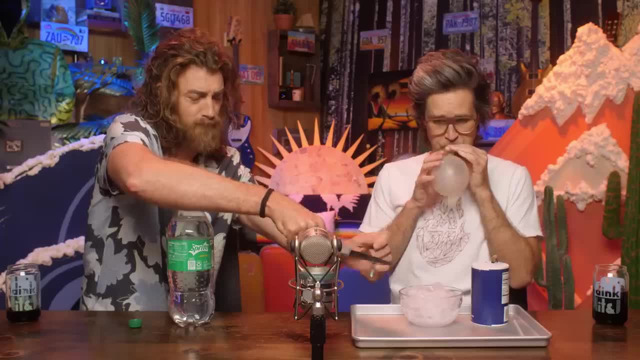 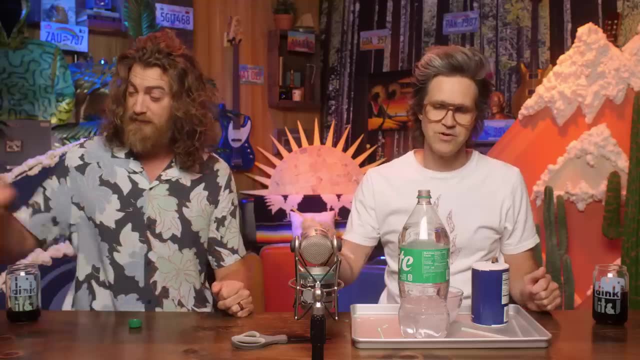 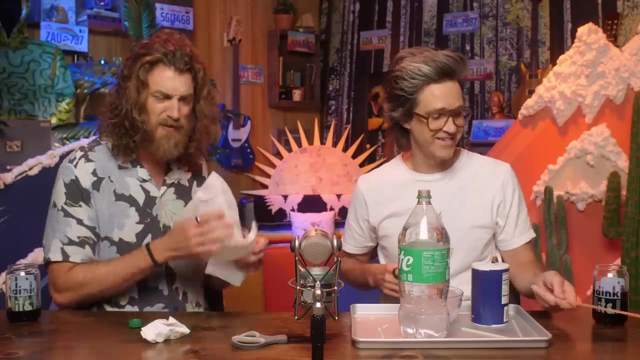 So I got something in my eye. Yeah, yeah, put it in there. We need a decoy. Do I need an eye flush? You do not need the glow stick. Oh yeah, All day long. Yeah, she was like. 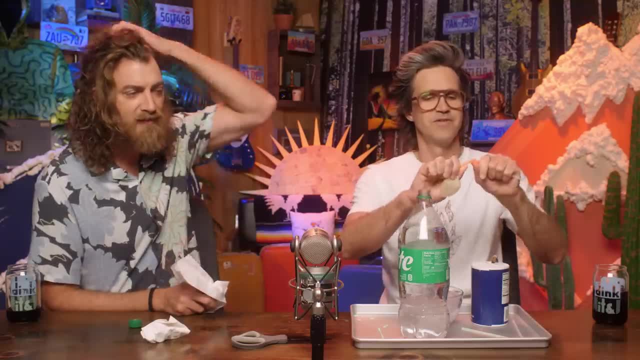 It's probably non-toxic. these days, Kids are crazy. Well, I was told to tell you don't get it on your skin and don't consume it. So you got it on your mustache and your eye, So in the eyes, all right. 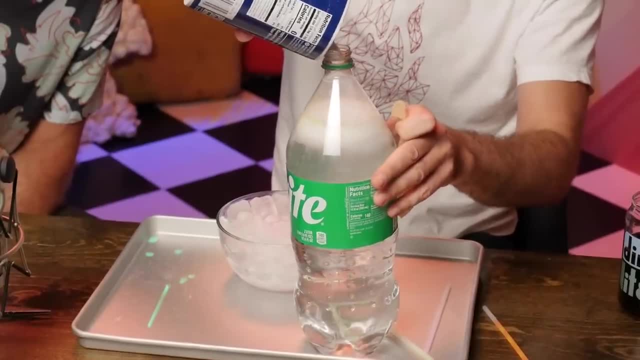 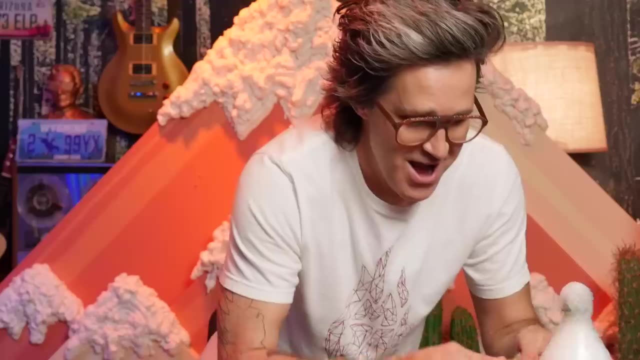 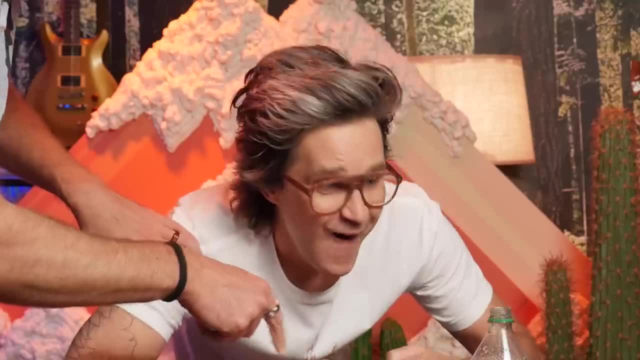 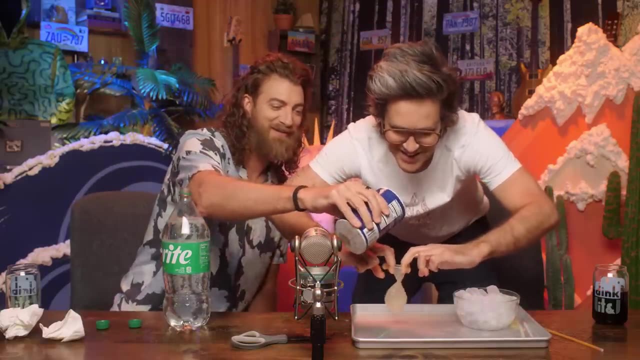 I figured it out. What Put salt in the balloon? Oh, I need you to put two fingers in there, make a big hole for daddy's salt And then turn that over into this. Okay, so, okay, all right. So you, at this point, you listen to me. 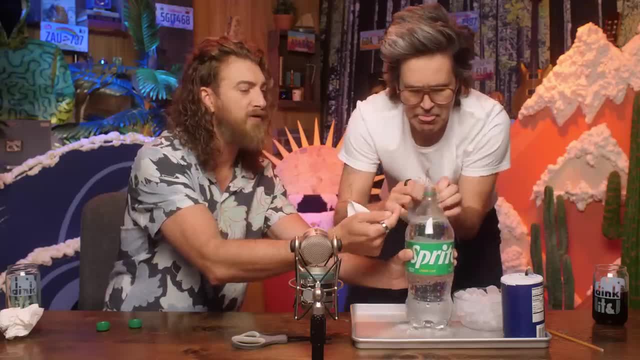 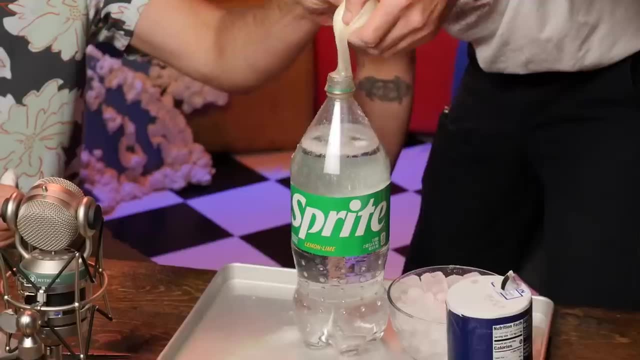 You put, so you put it on there without turning it over. You just get it on there, Don't get any salt in it, okay? So now, okay, now it's good. Then we just take this and we just lift it like this: 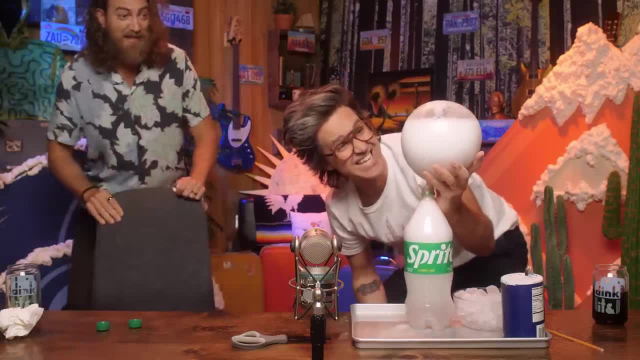 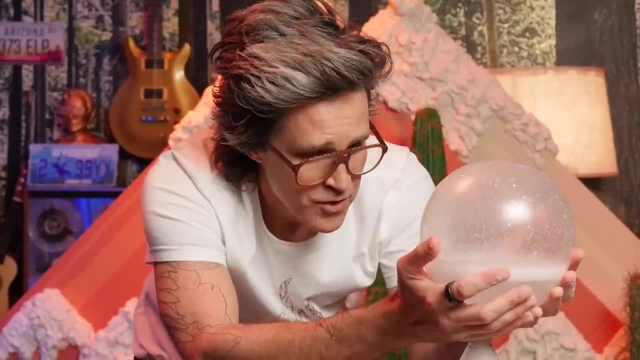 Look at that. Yes, Yes, It's gonna bust, It's gonna bust, It's gonna get all over the mic. No, Don't let it get on the mic, It's not gonna bust, It's not gonna bust. Oh, oh, look at it. 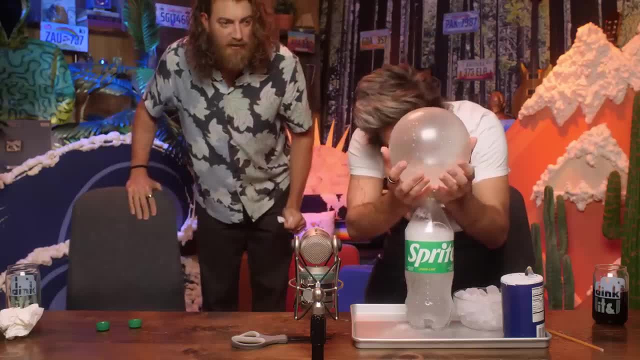 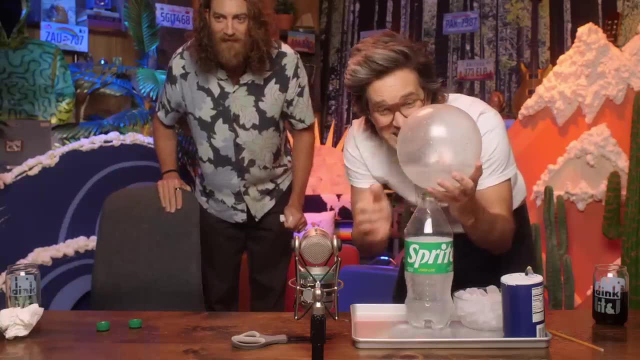 Oh, look at it. Oh, look at it. Look at what we did. And look, look, look. now there's bubbles. You hear that noise, The Beaker Boys, this is the sound of winning. We did it. 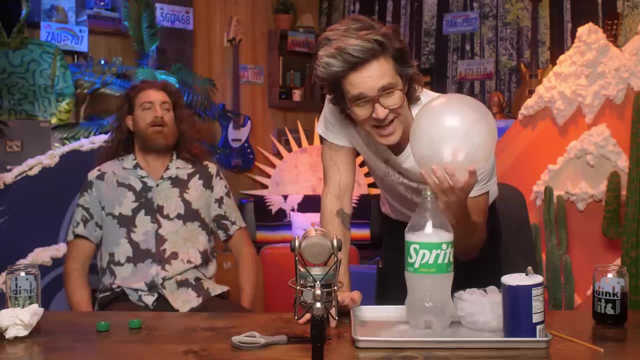 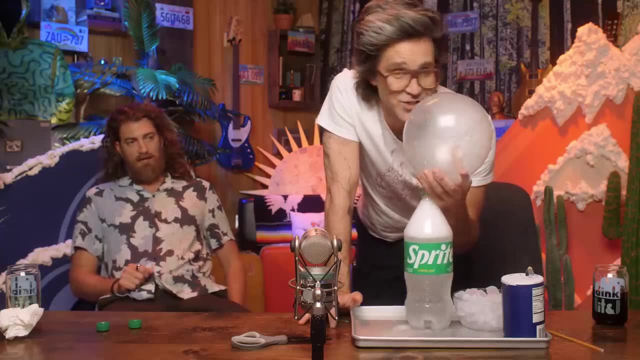 Did we do it, Man? I'll tell you. it came down to three points. I wanna thank Caitlyn for having such a good attitude, And I wanna thank Mikaela for being so darn cheap. Let's see them, Let's see, let's see. 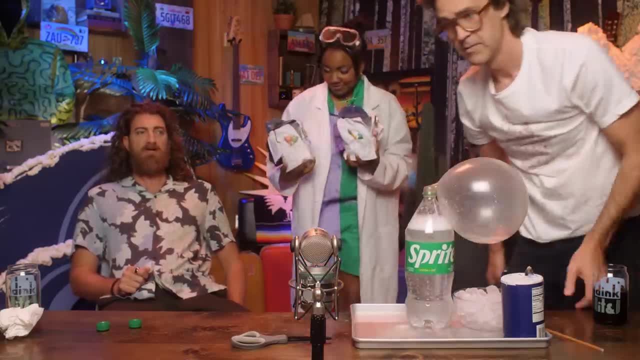 Let's see our prize, Let's see. Well, I wanna see if Caitlyn did a good job. I wanna see if Caitlyn did a better job than us. I wanna see if Caitlyn's balloon is bigger than ours. Oh, 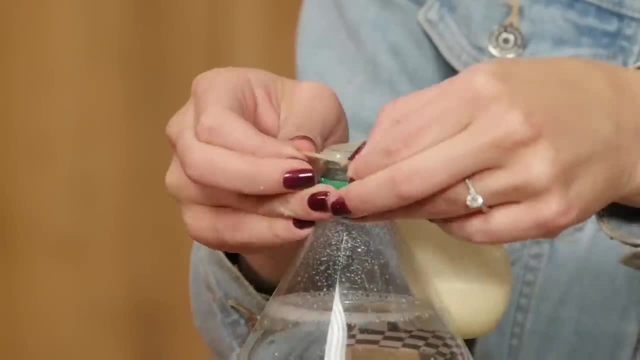 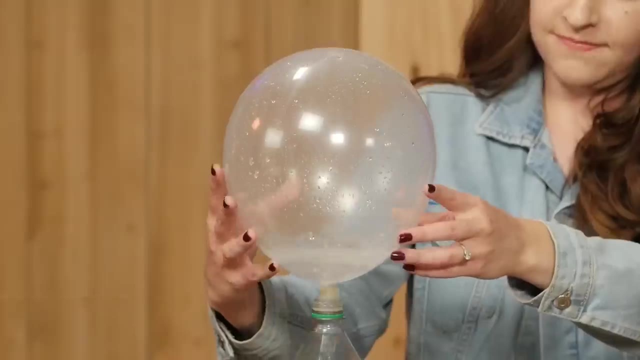 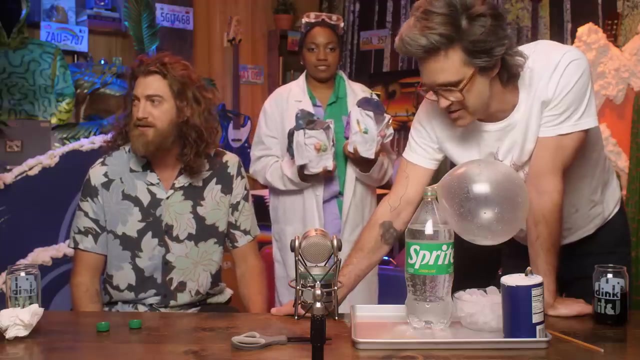 Children gather round Caitlyn, She's gonna make a balloon. good kick, Ooh, ooh. Little time ramp action. All right, we didn't need to watch that. We didn't need to watch that. She just made a balloon. that's a little bit bigger than ours. 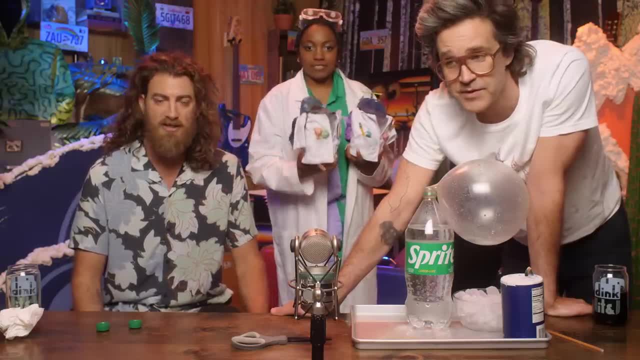 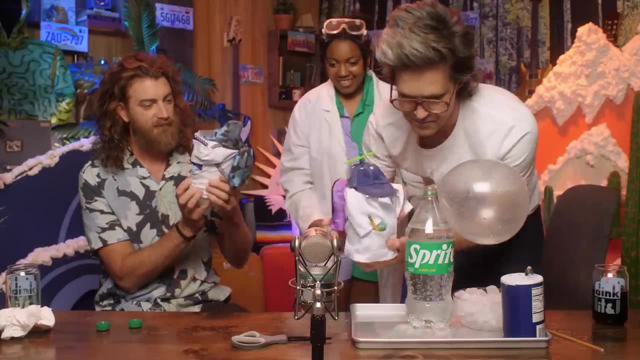 She did the same thing we did, with a lot more self-control. She looks so cute, She'd do it by herself. Oh, and look at these. Look at your little beaker boys. We're gonna take care of them. We're gonna feed them. 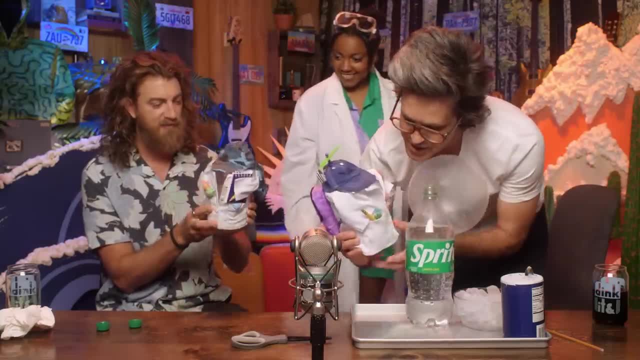 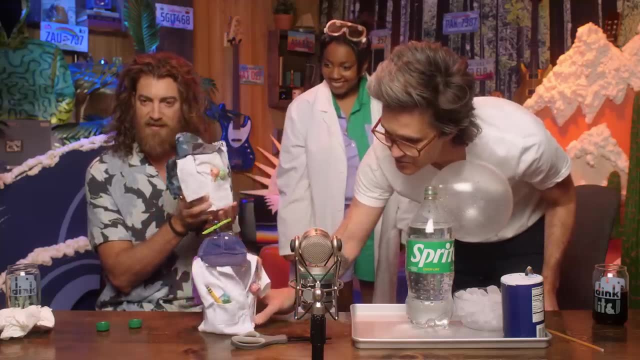 Treat them well. Those are my sons. Oh wow, It comes with a little dum-dums- Oh, look at that- And a little backpack. Is he going to school? That is so cool, This little beaker boy going to school. 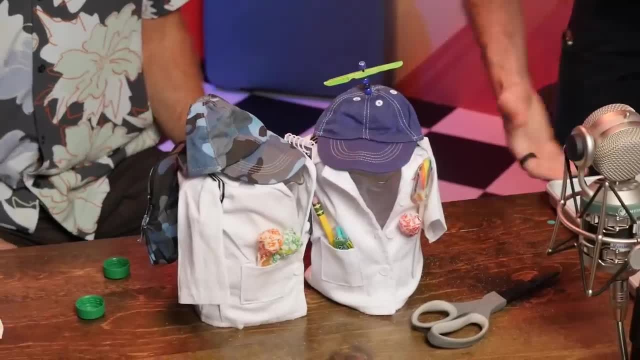 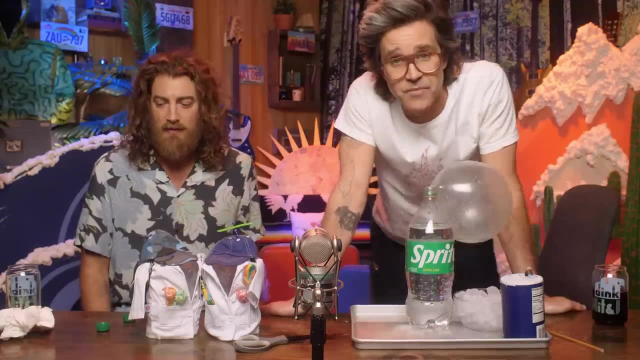 Look at that, He's gonna grow up. What's in there? Congratulations to us. We did it Link. We got three points to take home and spend any way we want Any closing praise. Praise, Stevie, You did a really great job. 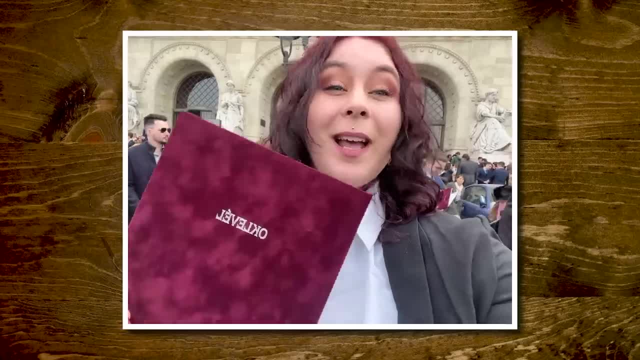 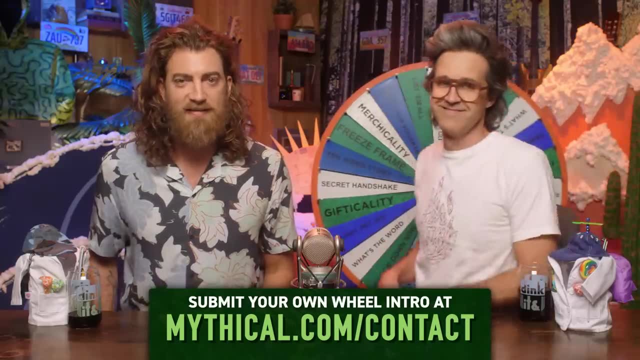 Thanks for subscribing and clicking that bell. You know what time it is. Hi, my name is Anita and I just got my engineering degree, and it's time to spin the Wheel of Mythicality. All right, you can now go be an internet star. 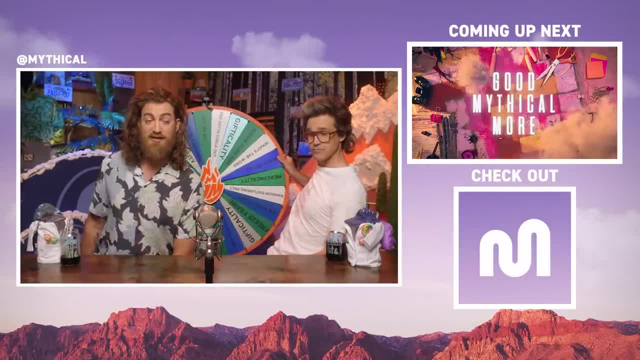 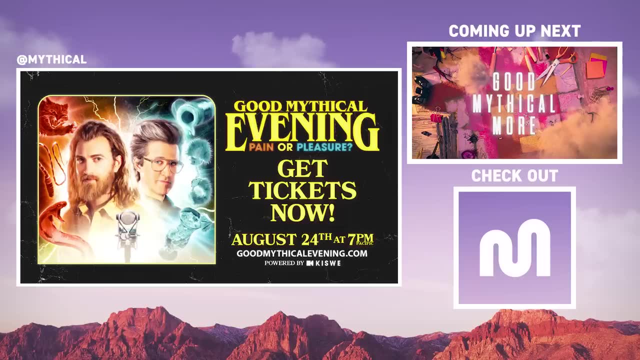 Yeah, Click the top link to watch us give 30-second science lessons in Good Mythical More And to find out where the Wheel of Mythicality's going. Good Mythical Evening is coming up fast. We are going live on August 24th. 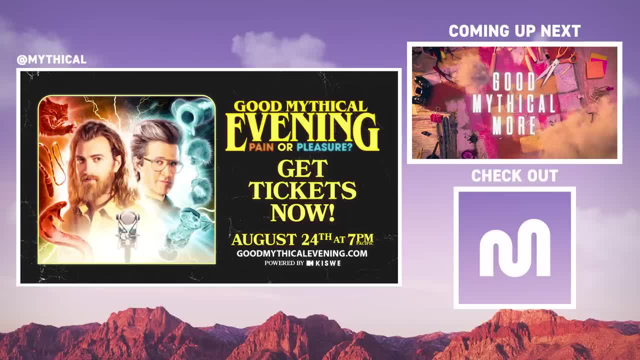 10 pm Eastern, 7 pm Pacific. so grab your tickets now at goodmythicaleveningcom.